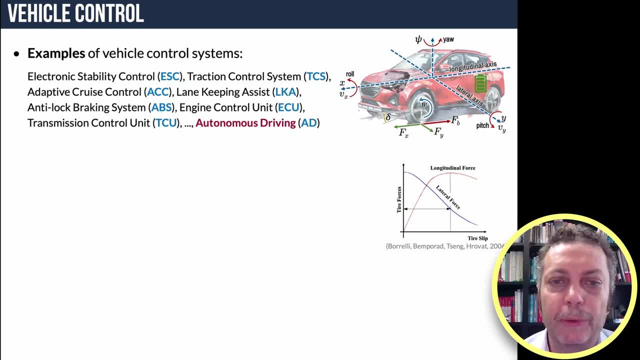 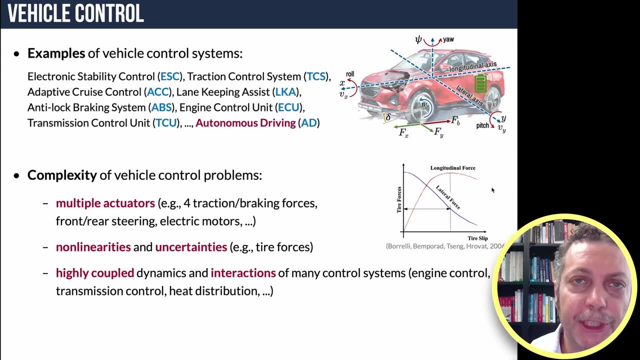 the highest level of control, if you want, that is, autonomous driving. So these systems involve different complexities, in particular, these sorts of complexities due to the presence of multiple actuators. For example, when you want to control the dynamics of the vehicle, you can actuate the four traction and braking forces acting. 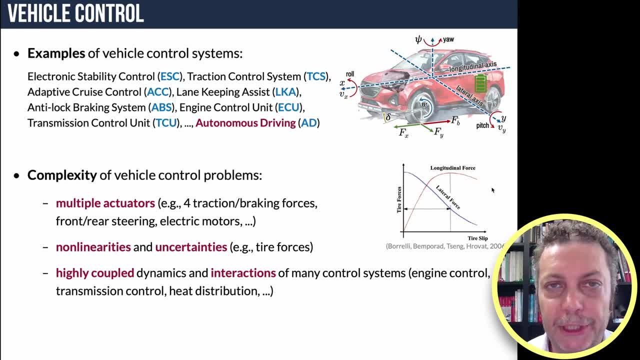 at different speeds. the wheels front steering, even rear steering in some cases, and also you may have electric motors contributing to the traction of the vehicle as well. So these are all actuators that affect simultaneously the dynamics of the system. In addition, the dynamics can be non-linear and uncertain. 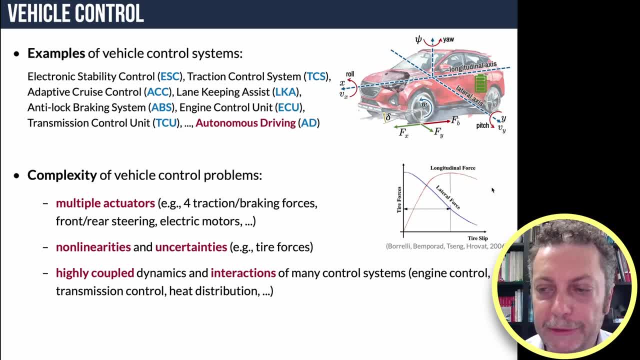 Again. think about the vehicle dynamics. the relation between tire slip and the resulting longitudinal and lateral forces are quite non-linear and also not very easily captured by models. And not only the dynamics are coupled, but also the different subsystems acting on the vehicle are interacting together. 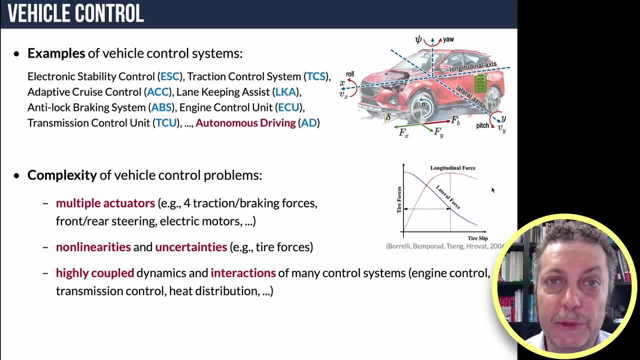 For example, the engine control system is related to the transmission control system, as well as to the battery management and even the heat distribution inside the vehicle. These are all coupled together. So control is a fundamental piece of software that can handle those challenges, that complexity. 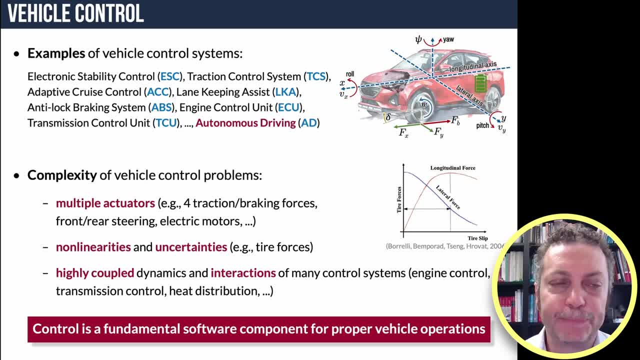 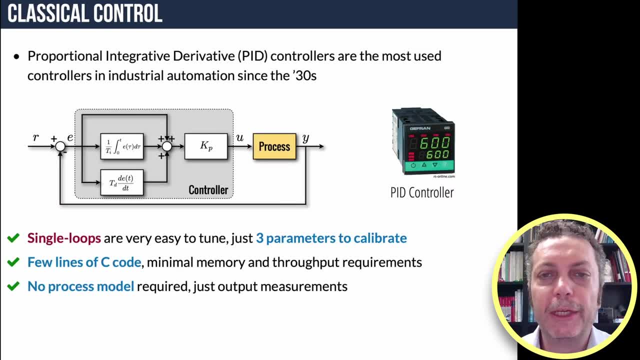 and ensure proper vehicle operations. There are many different control strategies one can use for designing vehicle control systems. Let me start with the most standard ones: classical control techniques, in particular PIDE control, which is still heavily used in industry, in particular in the automotive. 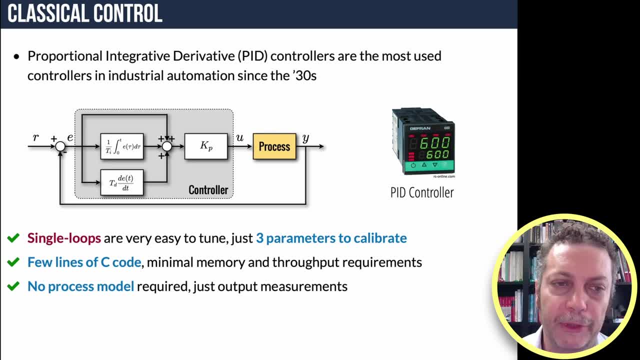 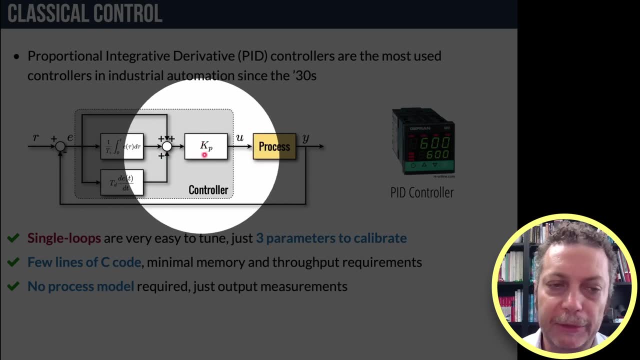 industry. And what is the advantage of PIDE controllers is that these are single loops. they are very easy to tune. Basically, you only have three parameters to choose: the proportional constant, KP for proportional error feedback, and also the terms TI, TD for the integral and derivative. 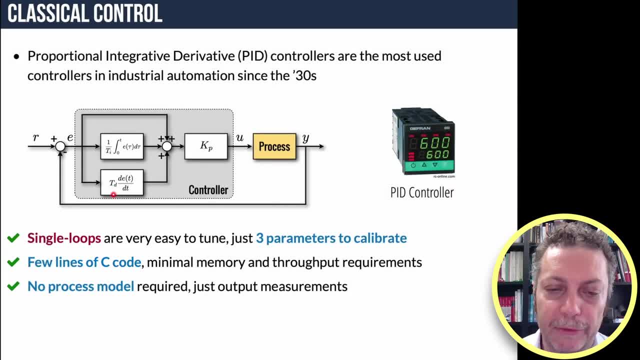 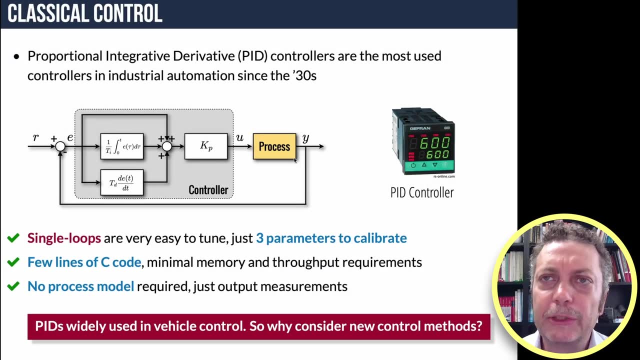 term, It can be implemented in very few lines of C code, doesn't take much memory and is fast to compute, And also it doesn't require to model the process explicitly, because it's only based on output measurements. Okay, so why then should we consider new control methods and more advanced control strategies? 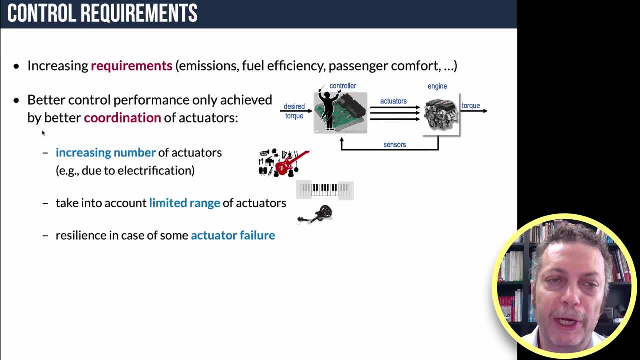 Well, there are a certain number of requirements- and increasingly stranger requirements- that you need to satisfy to design a vehicle control system, and a better control performance can be only achieved If you coordinate different actuators in a good way, hopefully in an optimal way. 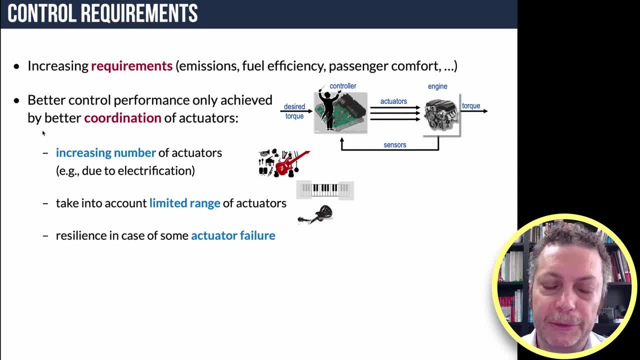 So the number, as I was mentioning before, the number of actuators is increasing. The actuators are limited, so you cannot decide arbitrarily the value of an actuator has, for example, if all is between zero and 100%, And also you want the controller to be resilient in case some of these many actuators fails. 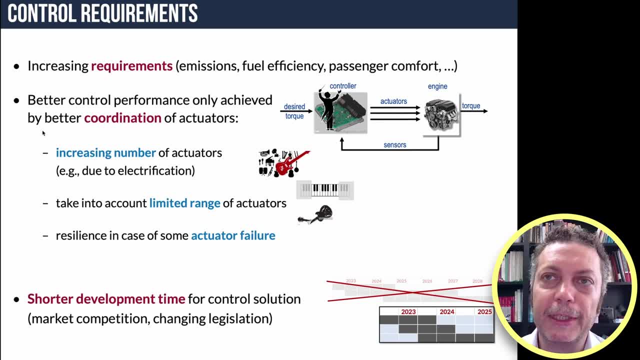 In addition to that, not only the problem is more complex, but also the problem is more complex. In addition to that, not only the problem is more complex, but also the problem is more complex. The problem is more complicated and more challenging, but also the time to develop. 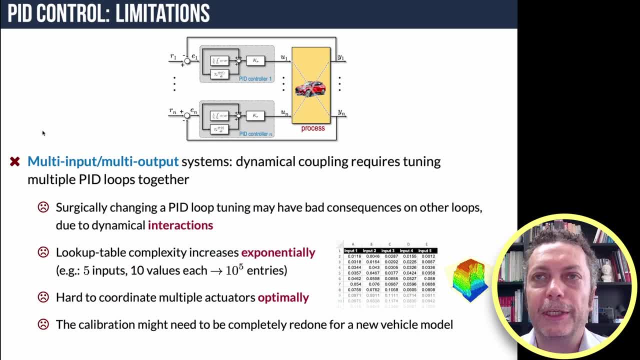 the controller gets shorter and shorter. That's why you need control strategies that can address those requirements, And the classical controls unfortunately have limitations and not much. if you have single loops, they can still be a very good solution, But when you have multiple input and multiple outputs interacting together, designing single 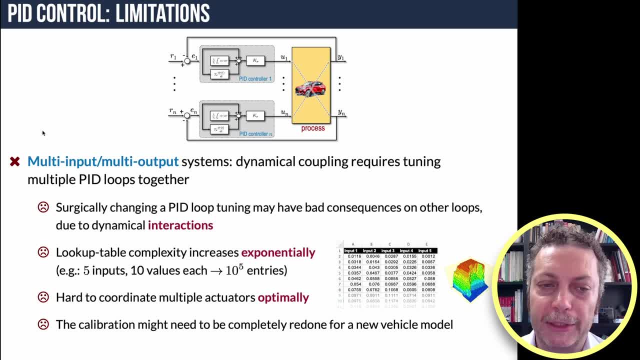 control loops and coordinate them can be quite challenging And, in particular, those loops interact with each other. So if you want to fine tune and change the parameters of one of those loops, this will have an influence on the other loops as well, due to the interaction. 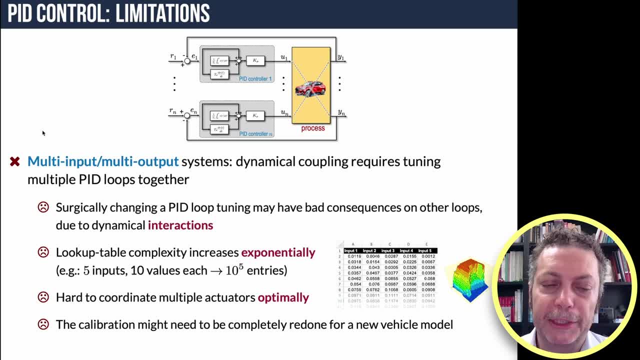 And often this is addressed by designing lookup tables. But lookup tables get more and more complex the more inputs that you have in the table. For example, if you have a lookup table for five inputs with 10 values each, it's already two to the power of five entries that you need to introduce in the table. 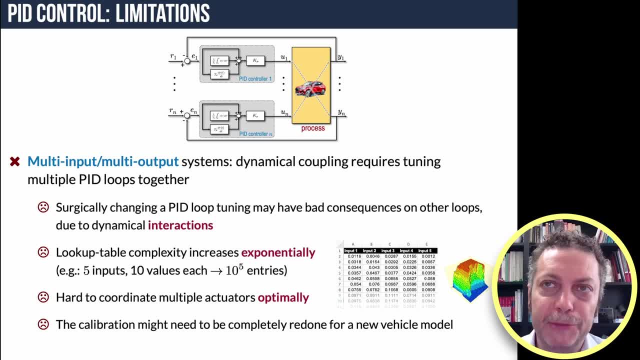 And you may come up with a scheme that works reasonably well, You're never sure whether this is optimal. it's actually often hard to coordinate those activities optimally according to a certain criterion And if you change the system- for example, if you have designed a controller for a certain. 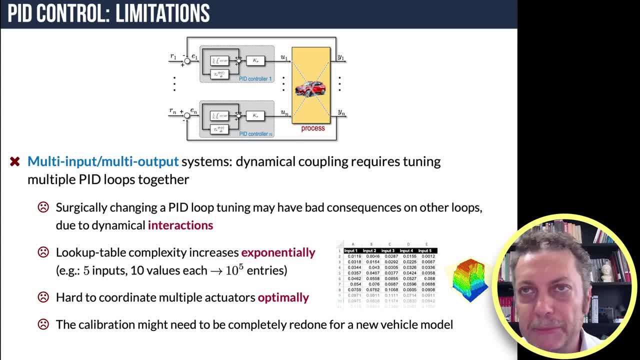 vehicle and now you go to the next vehicle, a new vehicle model- Maybe it's just slightly different, but it's different from the previous one- then you may need to calibrate again the controller and, for example, retune the lookup tables and the controller gains. 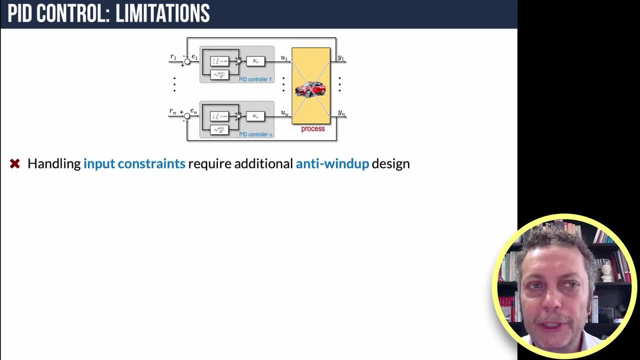 So this can be quite time consuming. Moreover, those more classical linear control schemes don't directly handle the input constraints, So you may have to add anti-windup scheme to make sure that the constraints are probably enforced. Output constraints are more difficult to 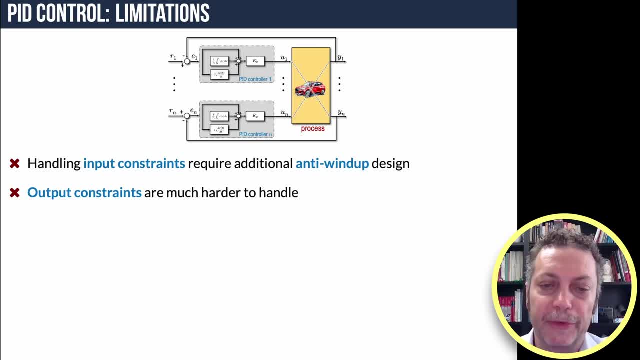 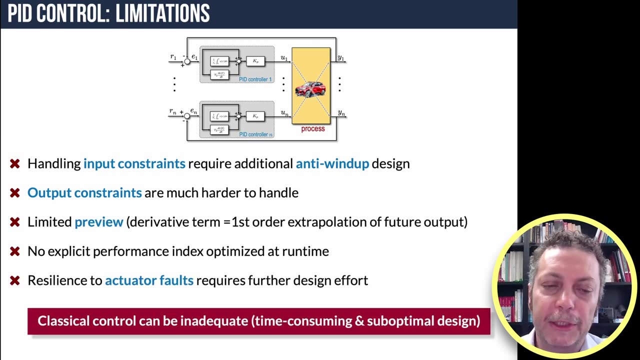 handle than input constraints. You cannot just saturate the value. You have to be careful the way you generate the actuator value so that the outputs of interest that you want to track the reference also satisfy certain constraints, so are within certain bounds. And if a certain actuator fails you have to design the single loop controllers so that 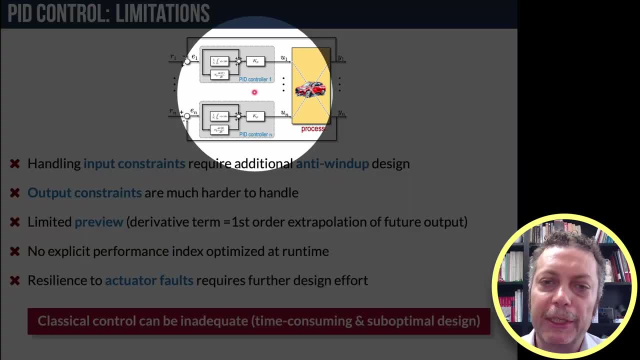 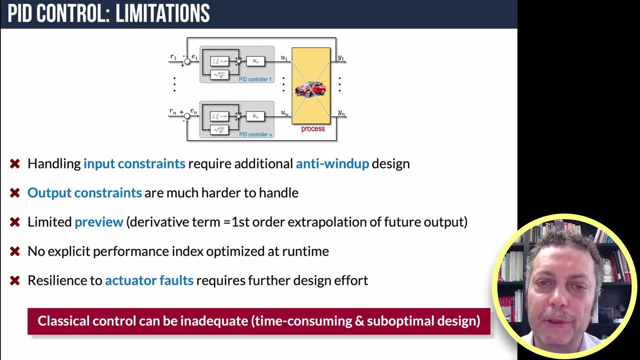 they work. also in the absence of some of the actuators. Then you have to make sure that for every possible configuration of the multi-input, multi-output controller, this works properly, which adds extra effort in designing the controller. So in many cases these classical control methods can be inadequate because they are 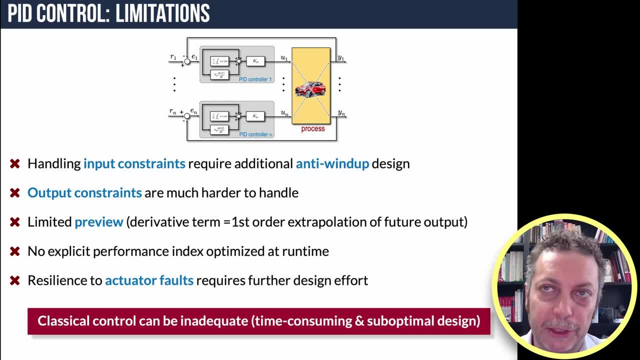 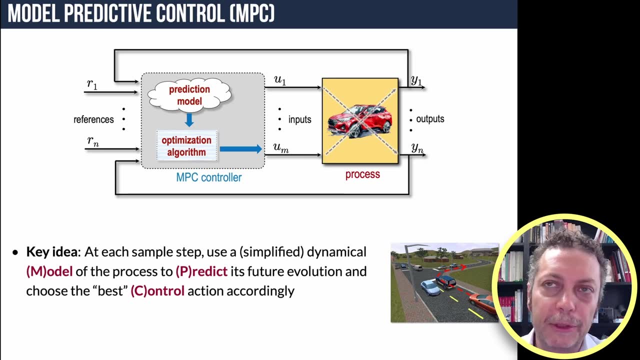 either not reaching an optimal design, so they don't ensure an optimal performance, or just because they are very time consuming to design and to calibrate. Now what are alternatives? Certainly, a good alternative is modern predictive control, which is the topic of my presentation. 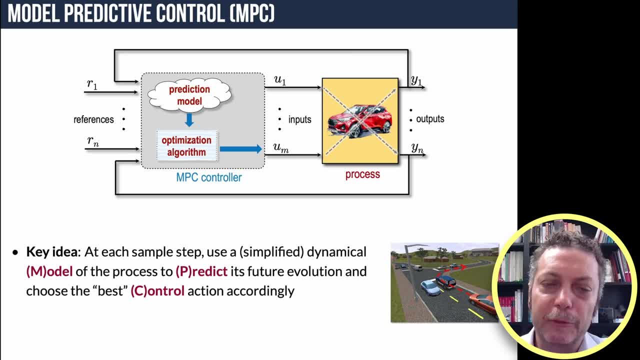 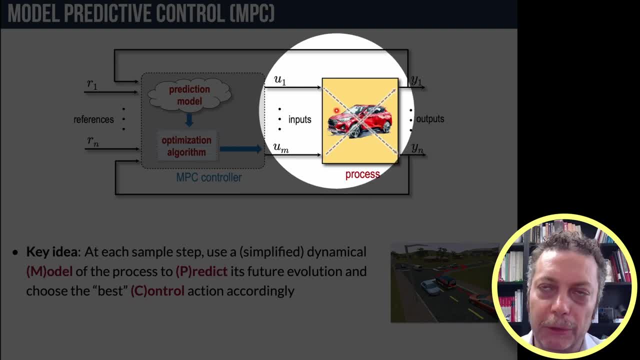 today. So the idea of MPC is, instead of breaking the multivariable control system into multiple loops, it handles the whole control problem in one shot. So the algorithm generates altogether a certain number of inputs so that a certain number n of outputs track the corresponding reference signals. 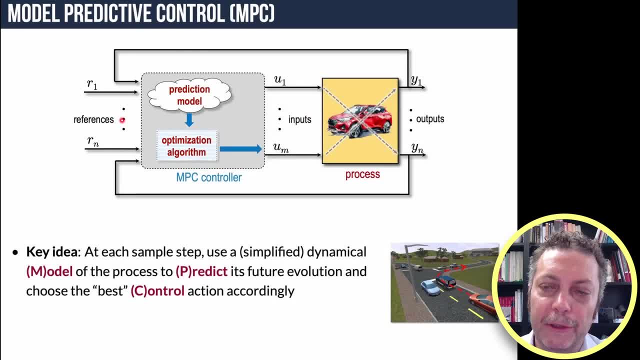 And it does this by using a model of the process that we are controlling in order to make predictions about the future evolution of the process. if you apply a certain sequence of inputs And among all possible predictions that can be done, it chooses the best one. 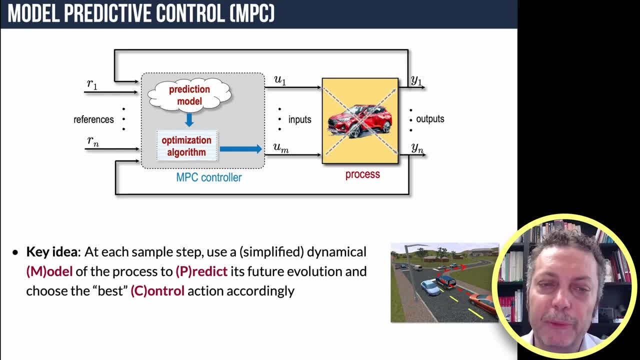 So it chooses the best sequence of inputs in the future. so in the prediction that optimizes a certain performance index. That's why it's called Modern predictive control: Exploiting a model of the process to make predictions about the evolution of the process. 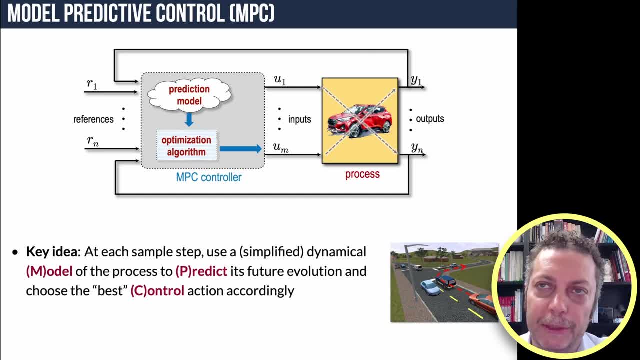 so that the optimal choice among all those possible evolutions delivers an optimal control action. Optimal with respect to, to the model. you have done so. if the model is not perfect, then it will not be optimal, but if the model is good enough it will be a good control action. 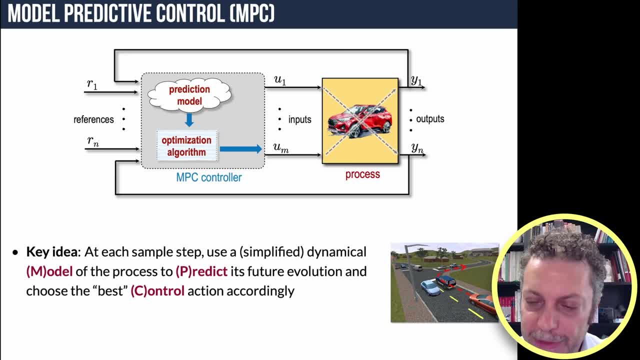 We'll come back on discussing about models of the process. We'll come back on discussing about models of the process, about model quality, in a second. So the idea of MPC is actually not very uncommon. That's actually what you do if you think about it. 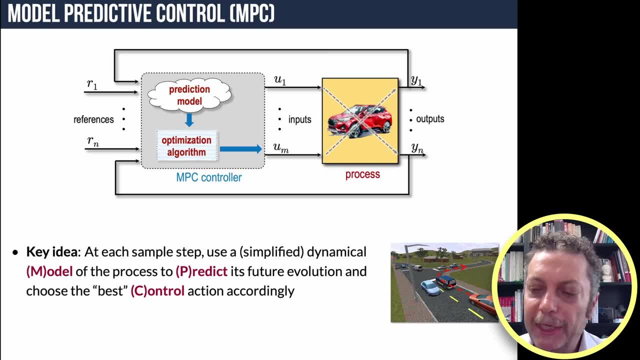 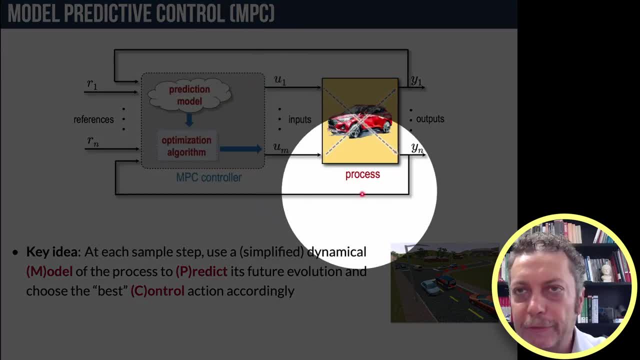 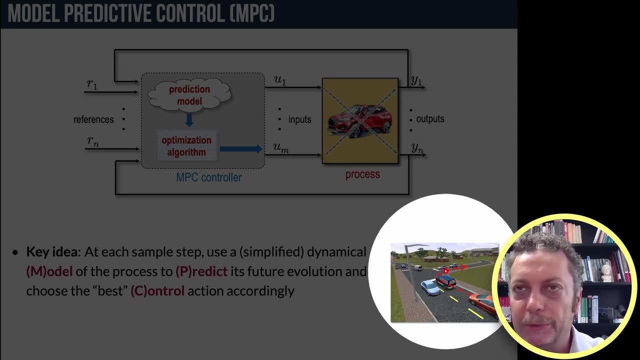 when you drive your car. When you drive, what you do is to look ahead at a certain horizon, in this case a certain space, for example, the next 50 meters. You don't have to look ahead the entire path between where you are now and where you want to go. 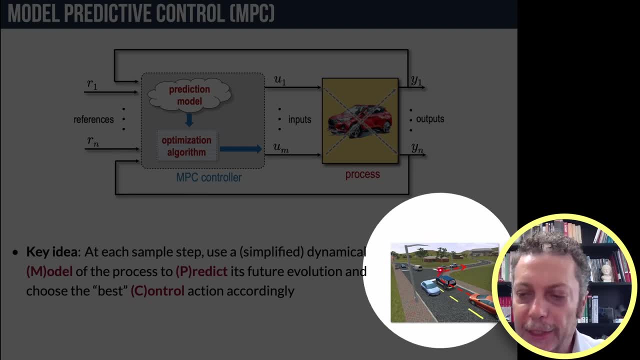 say, 10 kilometers away. just a short, close prediction. Okay, so the next meters, you want to travel, taking into account what is in front of you and around you. So the obstacle, the constraints on your, in this case, the constraints on your longitudinal position. 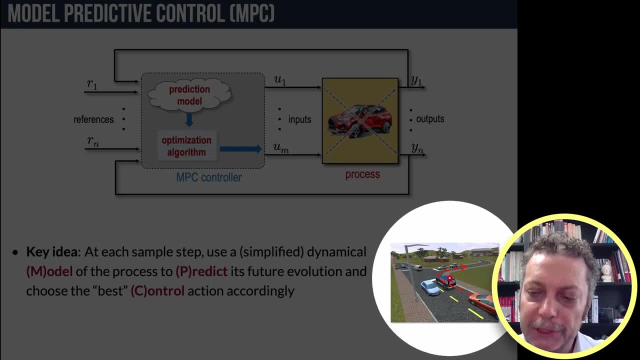 and then you plan a sequence of moves, So the way you want, for example, brake and steer your vehicle in order to turn right, And then, as you move, you re-plan continuously what you're going to do next. So, for example, when you have turned right. 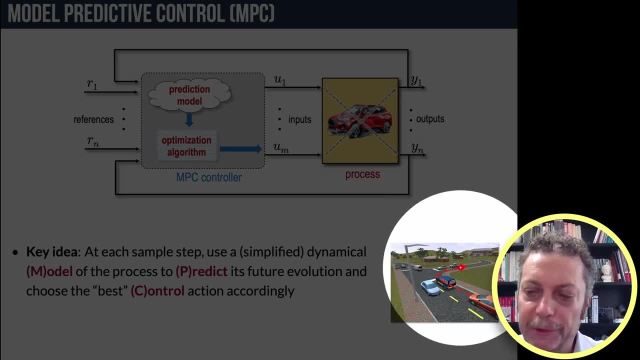 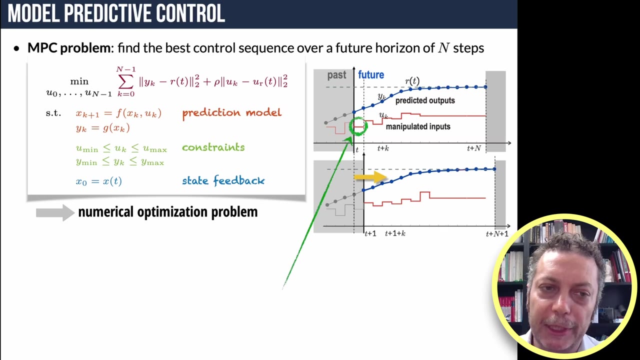 then you will forecast what happens between where you will be next and the next 50 or 100 meters, depending on your speed. That is exactly what is the idea behind MPC and, to state this more formally, let me introduce the optimization problem that MPC solves. 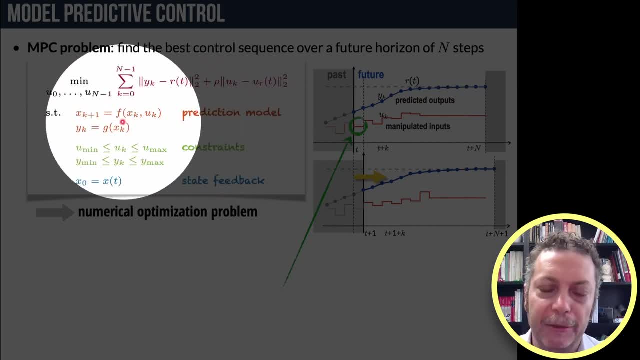 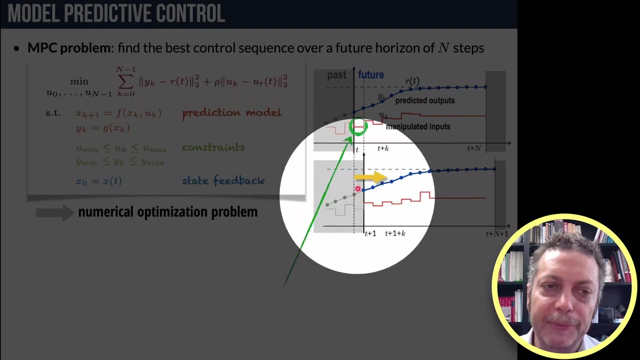 so the prediction model- the one here I like in orange color, is a very common problem for your vehicle- is a mathematical model relating the inputs to the outputs, to the states of the model of the system, and this model is used in prediction. so between the current time, say current time, t, which are 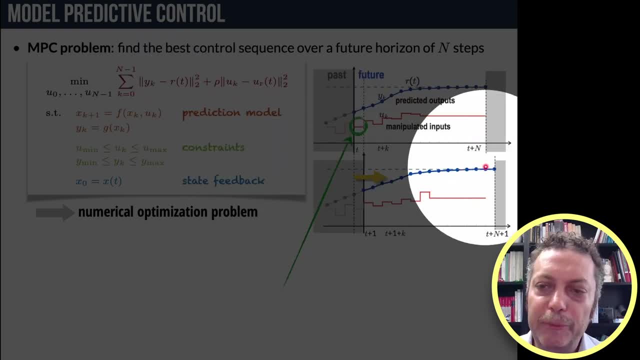 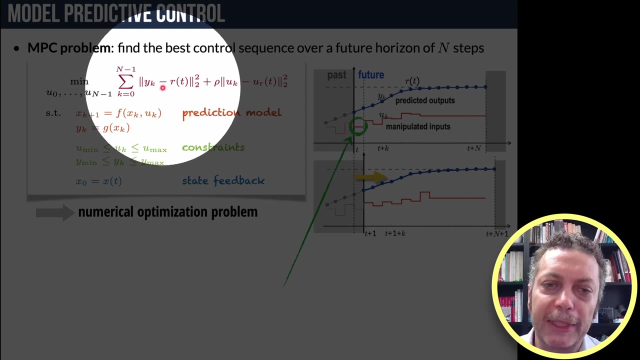 labeled as zero up to a certain time, t plus n in the future. okay, so you look over the future of n steps, what happens to the system according to the prediction, and try to optimize a performance index of different forms of the performance indexes you can use. for example, you can look at: 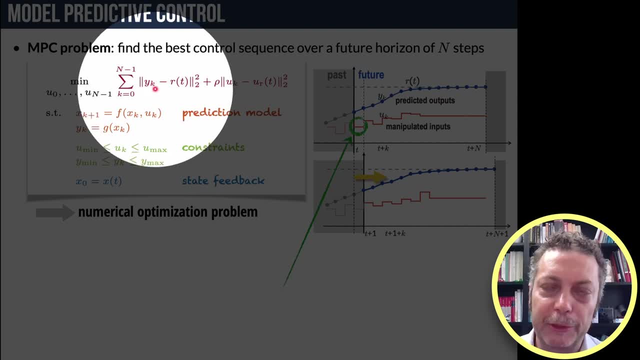 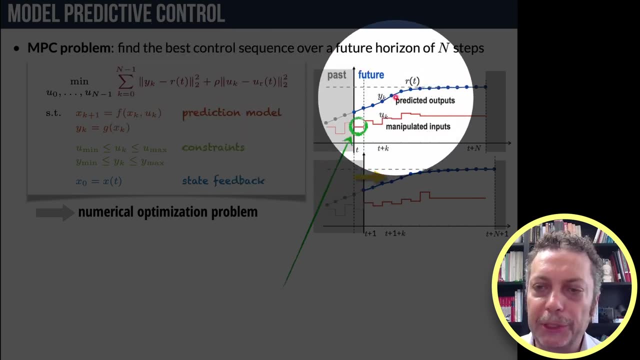 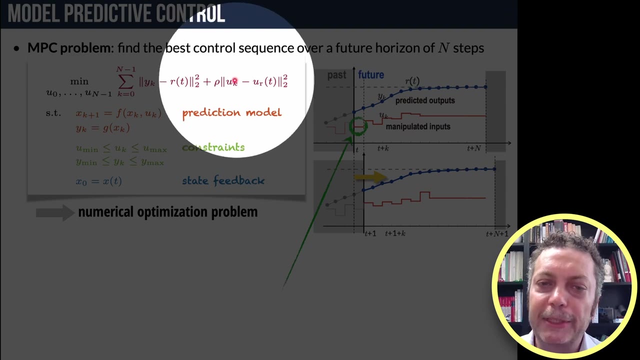 how large is the tracking error? so the difference between the predicted output and the reference signal you want to track. so this will be the difference between the two points you predict and the green signal, which is the reference. but also you may have some penalties on the inputs you apply and the corresponding optimal. 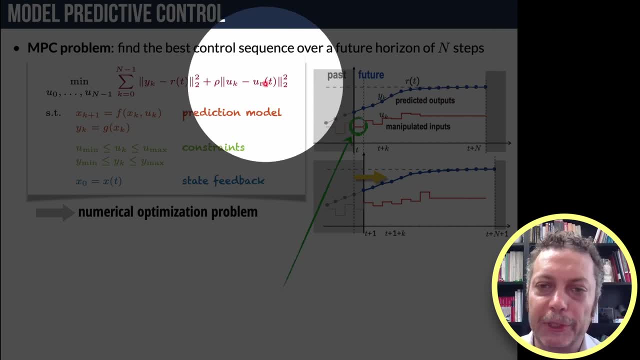 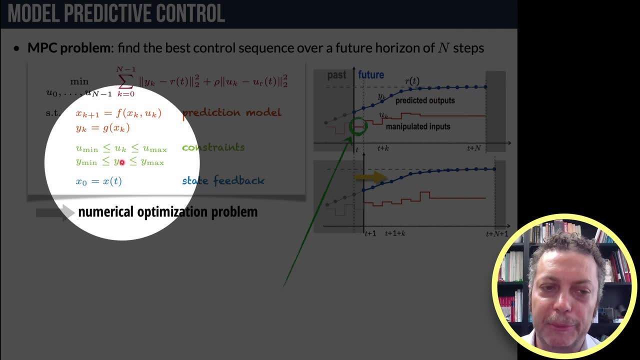 inputs that you would like to apply for the reference you want to track. so this is an optimal control problem. you can include constraints in the problem, so you may want to find the optimal sequence of inputs that minimize the performance index but that satisfies certain constraints. so the inputs in particular are between lower and upper bounds. 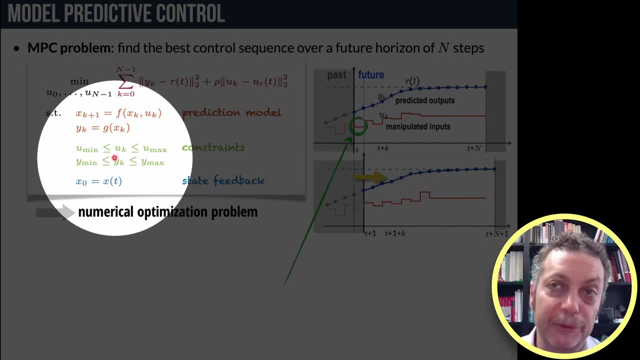 and the outputs as well must be. you can require that must be within upper lower bounds. so this is an optimal control problem that depends on the initial state, which is the current state xt where we are now. let's say, you can solve this problem by mapping the optimal control problem into. 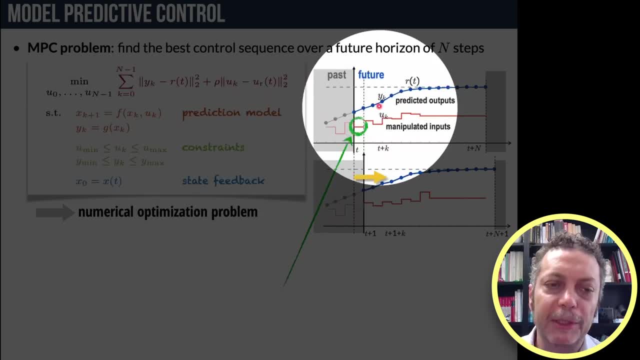 numerical optimization problem. you solve this problem. you will get a sequence of optimal inputs. now, rather than applying the whole sequence of inputs that you have computed, you only apply the first sample, the one highlighted here in the green circle, and at the next time, step t plus one. so 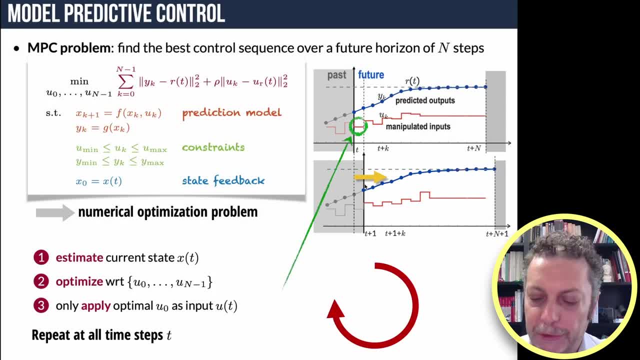 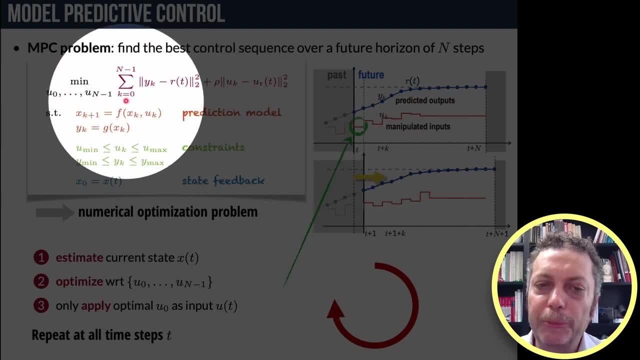 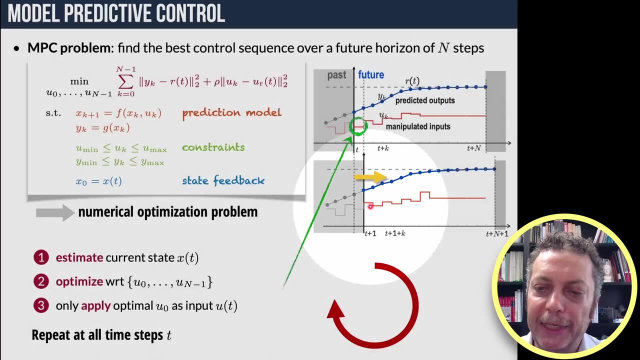 after one sample step you will repeat the procedure. so you will um get an estimate of the new state. xt plus one. uh, re-optimize the problem. okay, between time t plus one and t plus n plus one, get the new sequence, apply the first input and so on. so this is called the receding horizon mechanism, because the 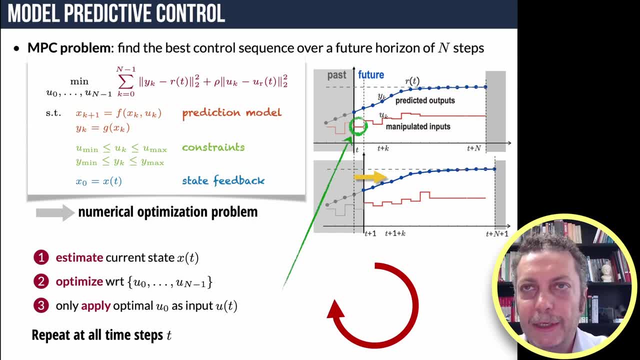 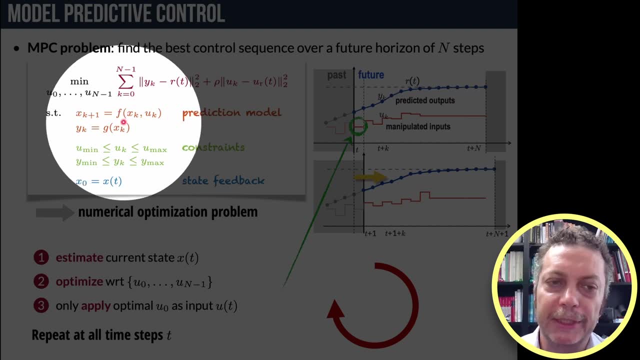 horizon over which you make the predictions and optimize receipts or slides over over time. so when the model is linear, so the model that you use to build the, the predictions, is a linear relation between inputs and states and between states and outputs, so given by linear state space. 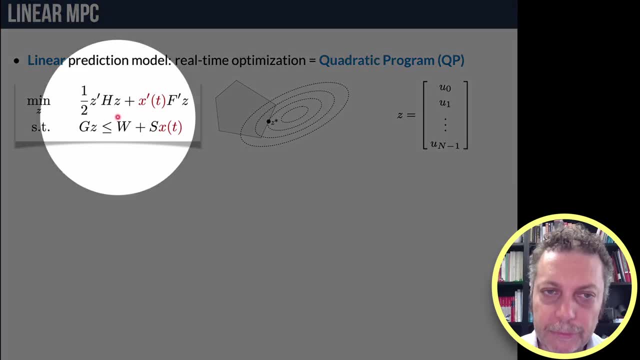 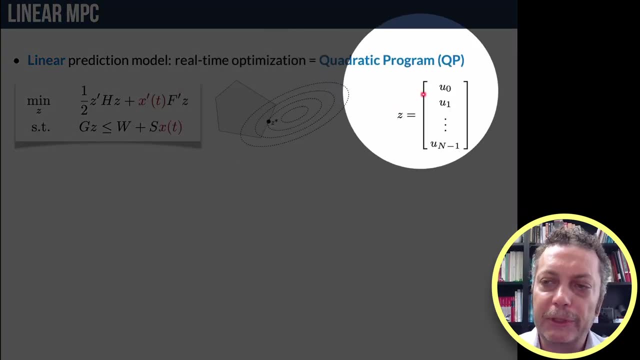 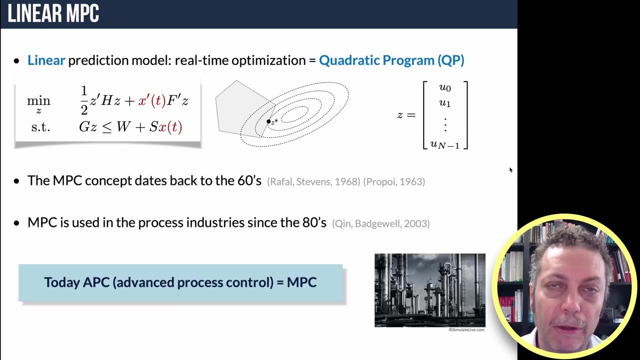 representation. then the real-time optimization pro you need to solve is a quadratic program with respect to the sequence of inputs. so let's call z the sequence of inputs. now the idea of mpc is not new, so the mpc concept date at least back to the 60s. 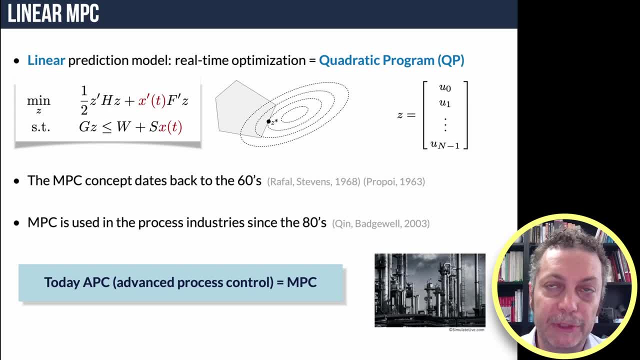 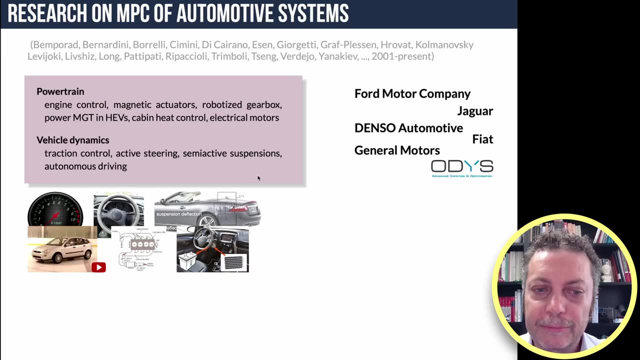 and, as a result, mpc is used- i'll say routinely- in the process industries since the the 80s and in the 1980s and so on. so what you need in a process control is called apc. advanced process control actually means modern predictive control. now regarding applications of mpc in the automotive. 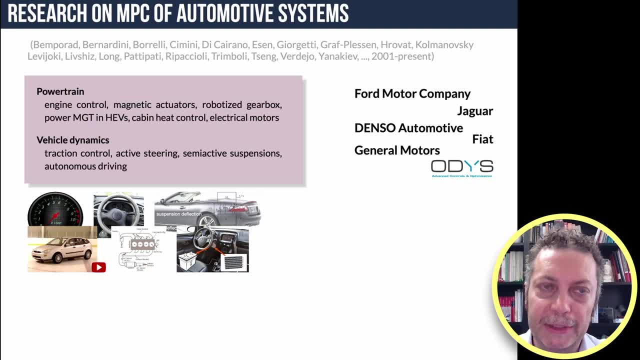 domain. a lot of research has been done um over the last decades. it's not only us. there are many, many groups um, both in academia and the industry that have been looking at research projects. uh, using mpc. Nowadays, I would say most, if not all the automotive OEMs, entire WAN suppliers, are looking into MPC solutions. 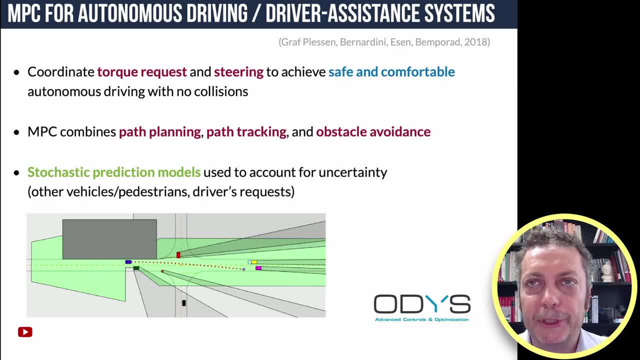 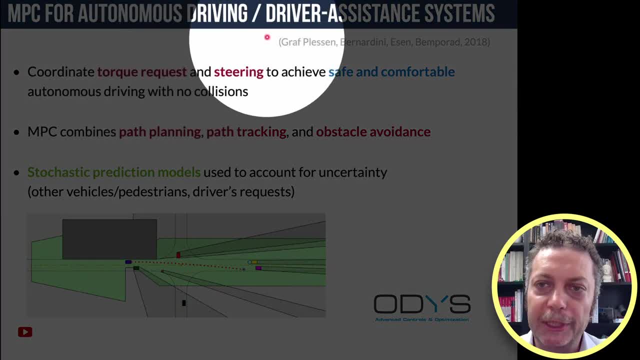 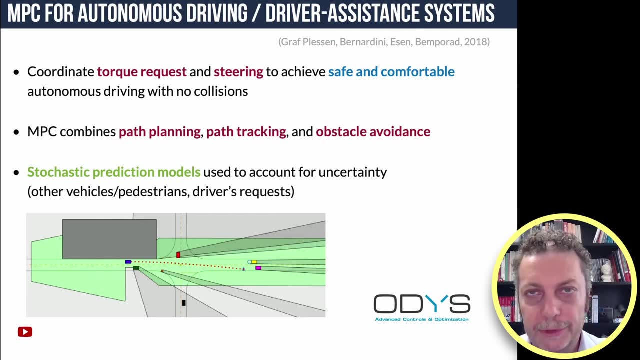 Let me mention one particular application which is particularly popular these days, often attacked by MPC ideas. This is also a problem where I've been working in the past, So it's autonomous driving, where the control goal is to coordinate torque request and the steering of the vehicle. 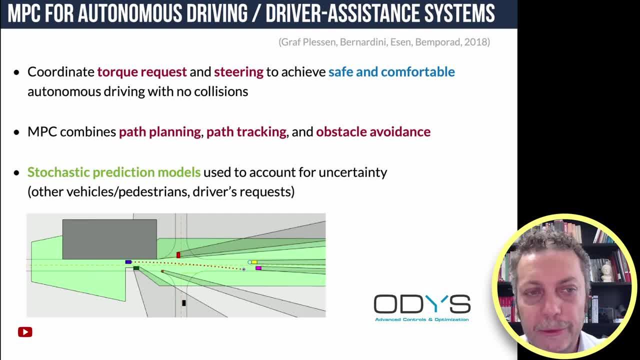 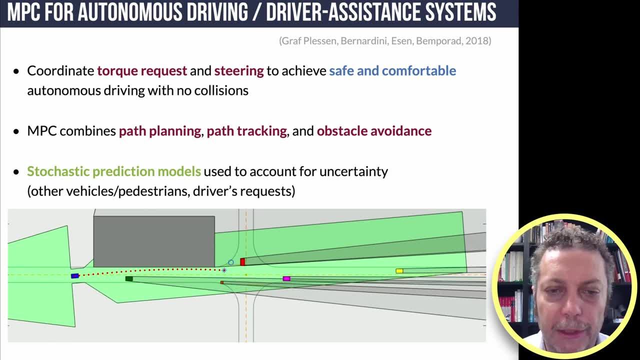 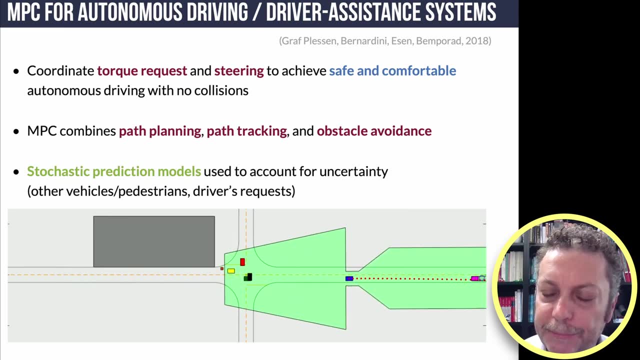 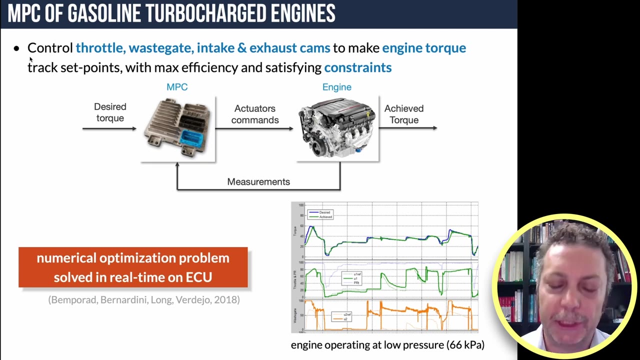 so to achieve a safe and comfortable drive, of course avoiding collisions. So let me show you an animation of the controller in simulation. So the red dots are prediction steps in space. Let me mention another application of MPC for controlling gasoline turbocharged engines. 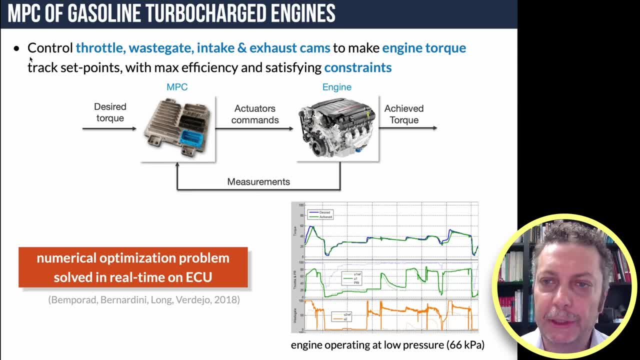 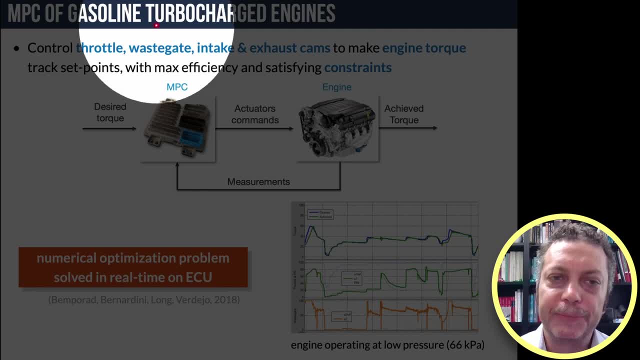 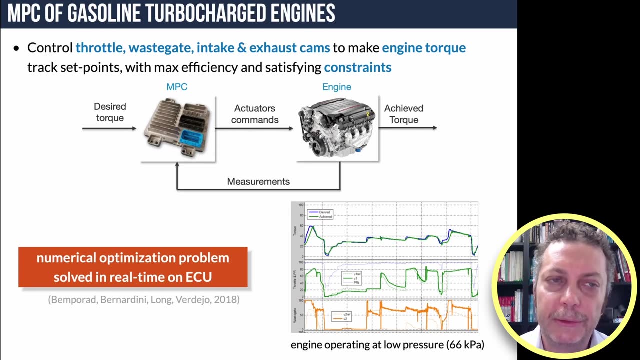 In this case, there is a single output, which is the engine torque you want to achieve, and you have four actuators, four inputs: the throttle wastegate bolts and the intake and exhaust cams. So you have four inputs to manipulate in order to get the desired torque with maximum efficiency. 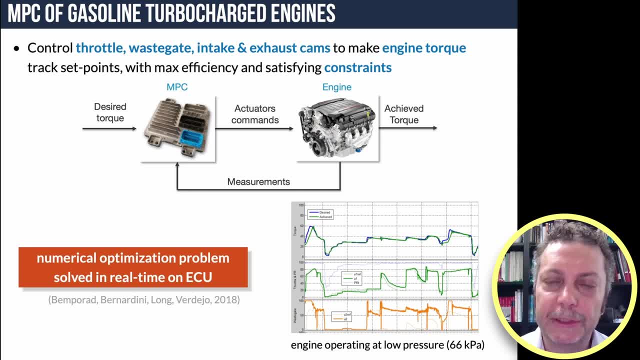 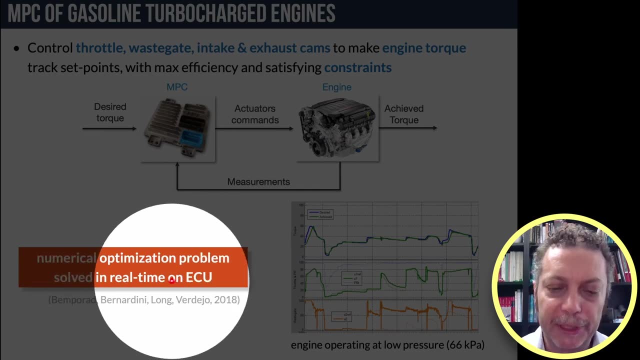 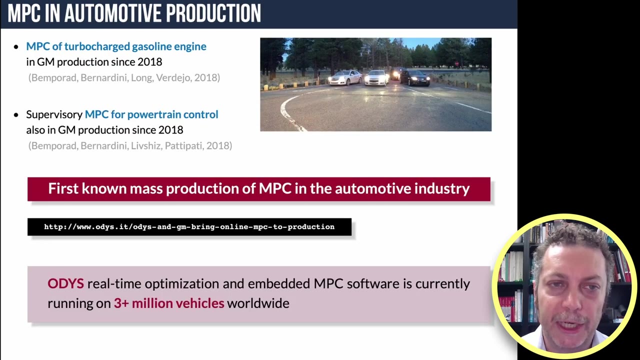 while satisfying constructions. So you have one output for movementкоangulation and one for steering. To achieve a certainly humming It will be possible. or you know it will take the power car to the getting to the power car, and so it will be possible. or you know it will take the power car but only selling the vehicles. Now, after the sound effect that make it much easier to get the driver, and but okay, good, We have a show that shows how H trabajar intra- holy warning lights, the transmi function of a machine that will motivate you to laughing- works. This honorable, essential control operation will work in the application that it embodies. It will be partially appropriate in this application. That's why we have in trade- it'll fill out- a wide array of computers that are very them. bicycles that shooting know that at 4 to 4, this is how they steVideo the first video such as this has. aber~ this is how you'll integrate brakes into the system. 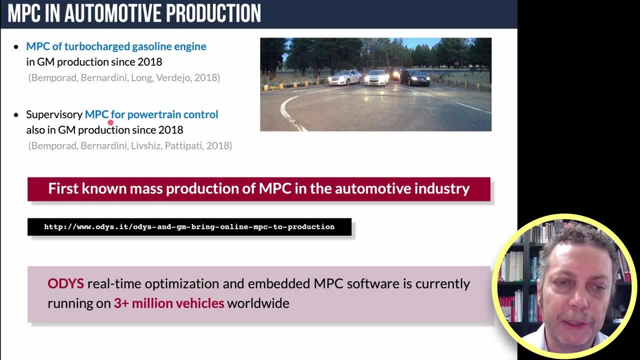 for powertrain control using CVT. So these are both in production and in mass production And, as far as we know, this is the first at least documented mass production of MPC in the automotive industry. And let me mention that all this MPC software is running nowadays. 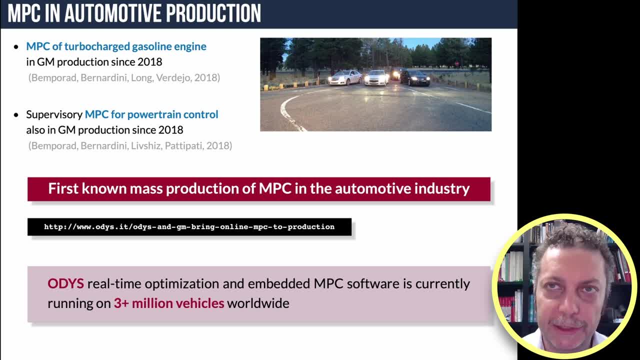 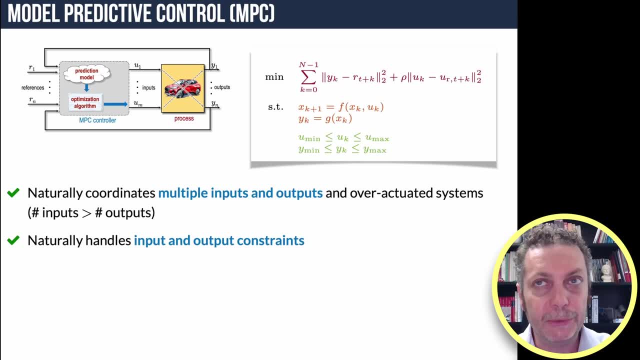 on more than 3 million vehicles worldwide in different applications. So what are the advantages of MPC? So why MPC is used and why many automotive companies are attracted by MPC. As I was mentioning before, this is one controller for the entire multivariable system. 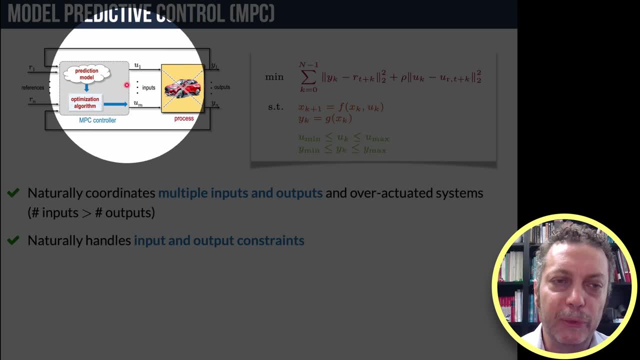 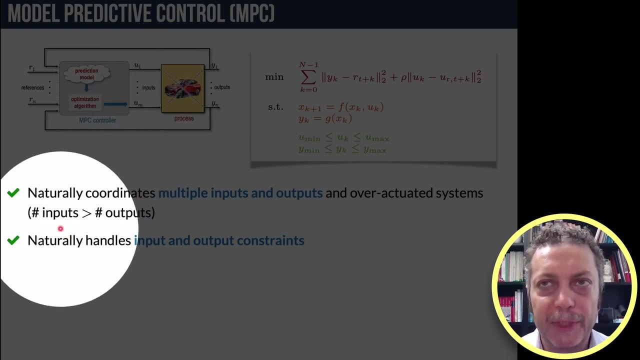 So it spontaneously coordinates multiple inputs and multiple outputs by solving one single optimization problem, And you don't need to have the same number of inputs and outputs as you would have if you have single loops. Actually, for example, the number of inputs as the engine control system. 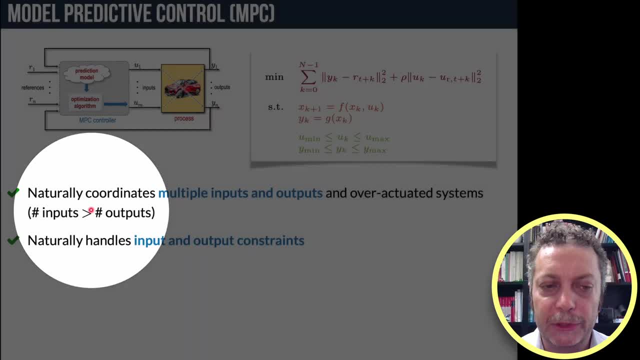 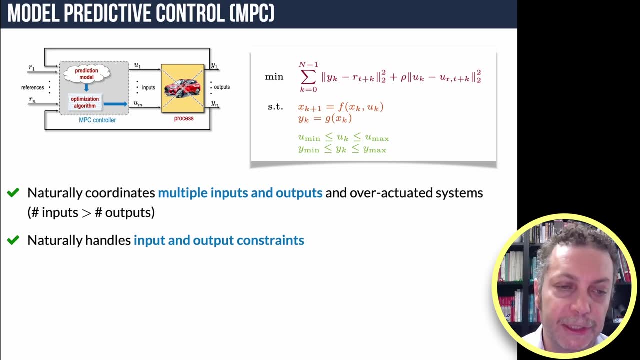 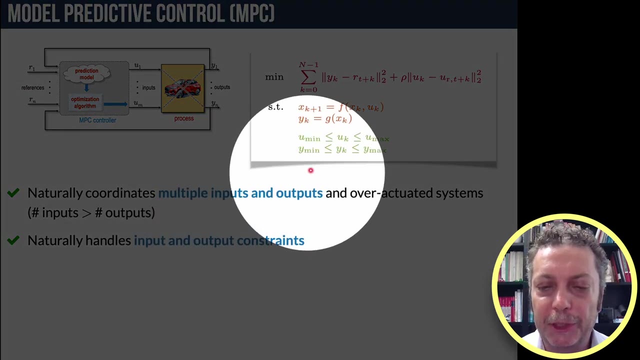 we've seen before, can be larger than the number of outputs. So you have to allocate the actuation action optimally and multiple combinations exist that gives you the same output. you want to find the optimal one. It naturally handles constraints on inputs and outputs. 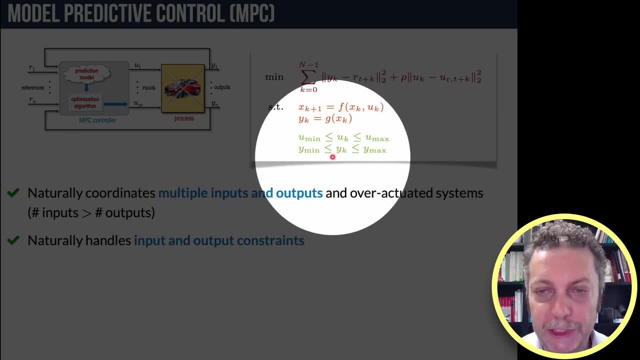 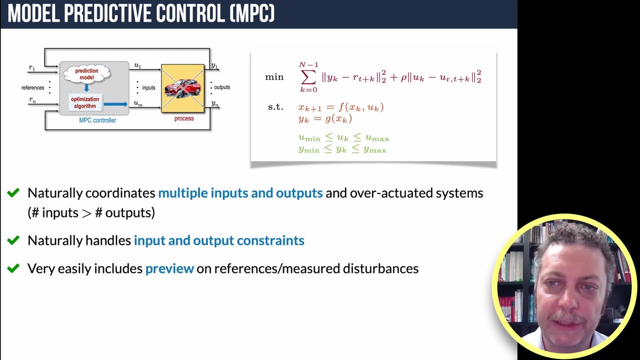 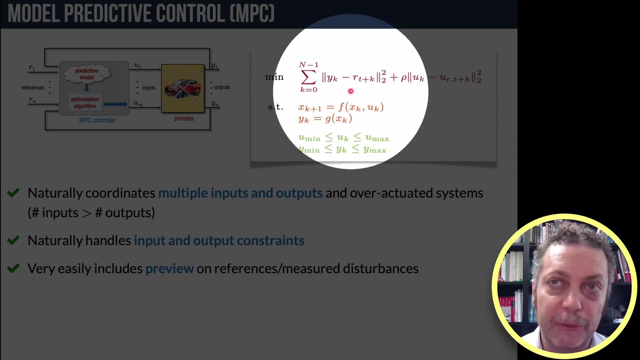 You just specify those constraints in the problem formulation. Those will be satisfied. You can include preview on the reference signal. You just plug in the samples of the reference that you know in advance and the optimization will depend. The result of the optimization will depend on those references. 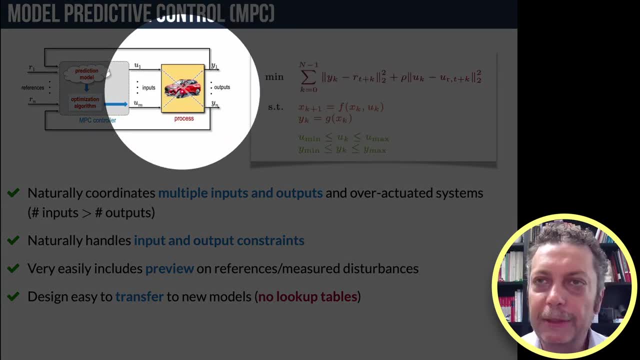 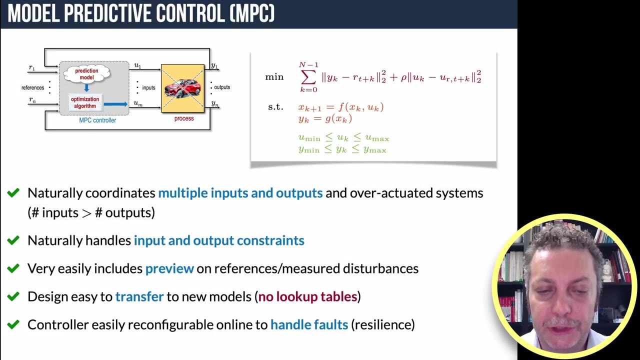 And once you have a design done for, say, a certain vehicle or a certain engine or a certain component of the system, then it's usually quite easy to transfer the existing design to the new model, And not only that, but also changing the configuration around time. 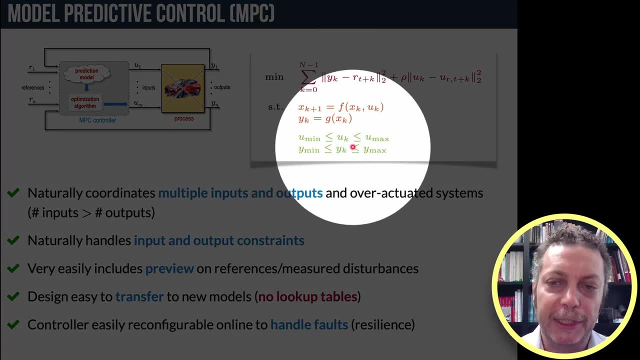 is actually very easy because, say, an actuator is stuck at some point, then you can just change the constraints: say u-min equal u-max, say equal zero, So when that input is not available, So the controller will reconfigure automatically. 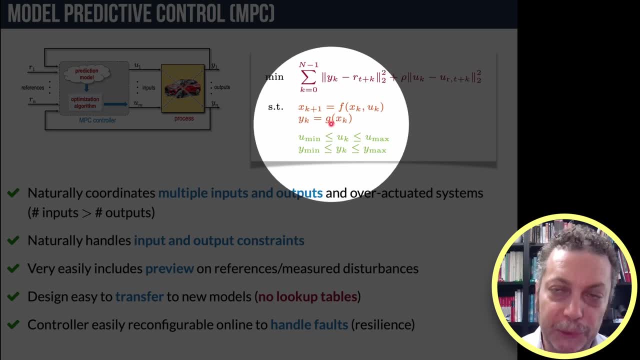 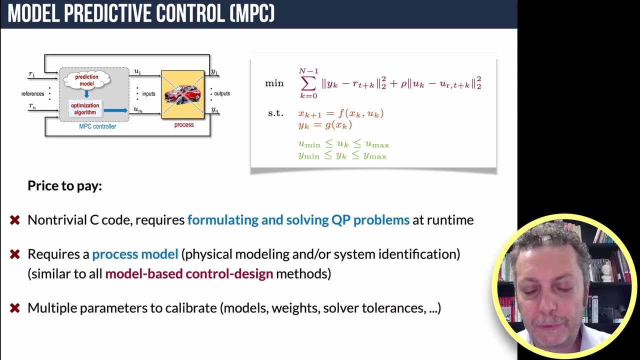 because the new constraints will be taken into account in the new optimization problem solved, since now It's now on. Now there are some prices to pay. First of all, the code to implement the controller is no longer as simple as PID, control laws or other type of classical control. 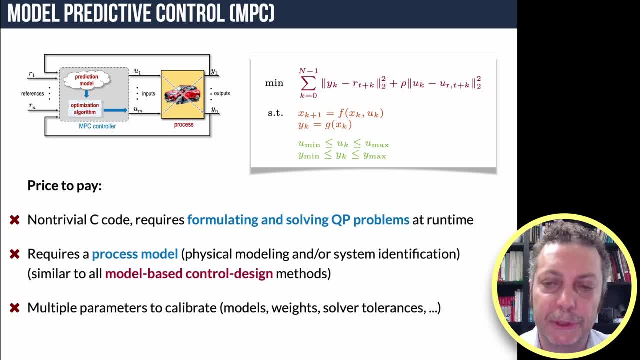 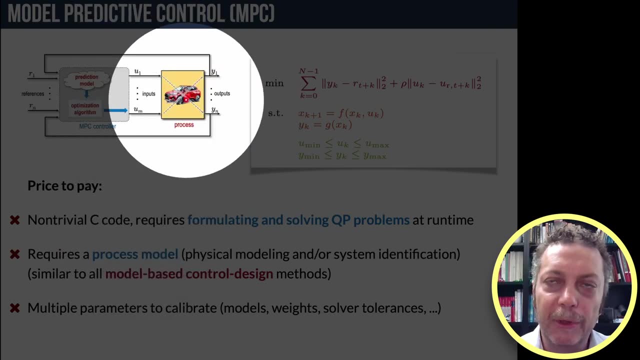 So you need to formulate and solve the QP problem online. So the code for constructing and solving the problem must run on the board. It requires a process model. So you need a prediction model. So you need to model the process you are controlling. 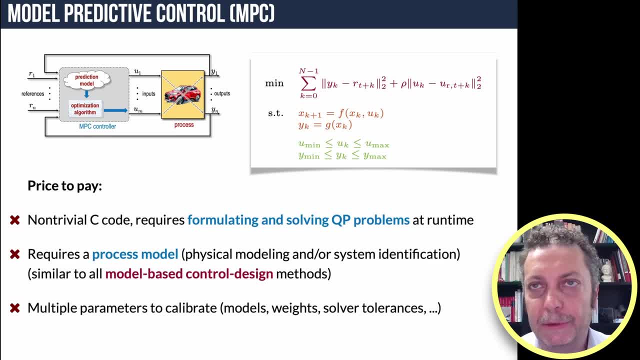 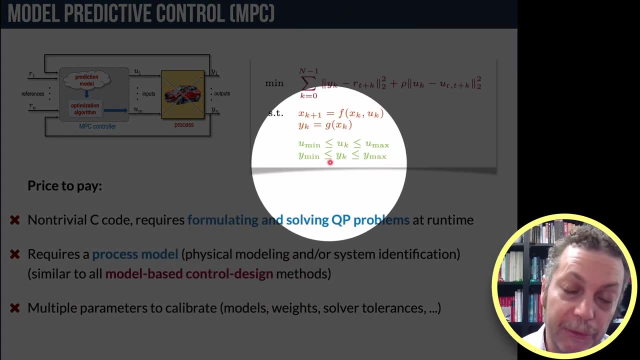 And this, by the way, is for any model-based control design method, even LQR, But also the number of parameters now to calibrate can be quite large, meaning you have to calibrate the weights also, the constraints Also. the constraints often come naturally from specs. 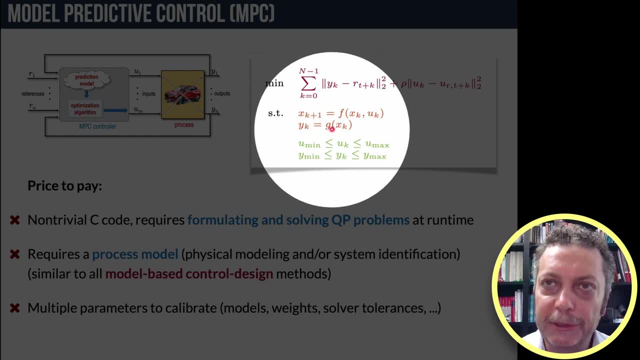 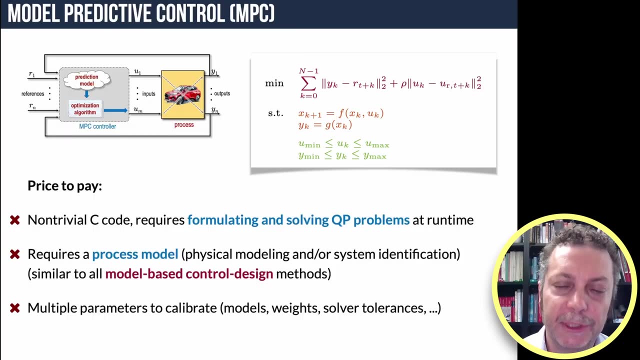 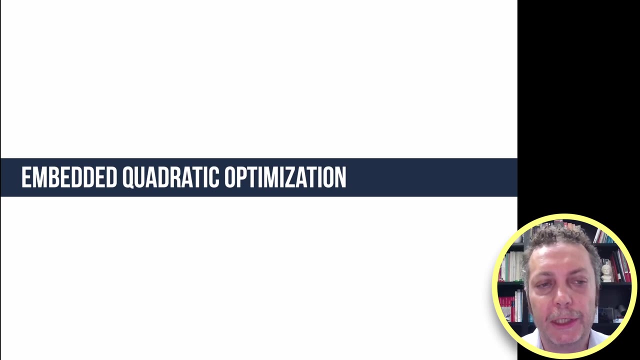 And in particular, you have to calibrate the model, So you have a degree of freedom which is the model itself. So we will see how to address that item in the remaining part of my presentation. Let me start with embedded quadratic optimization. 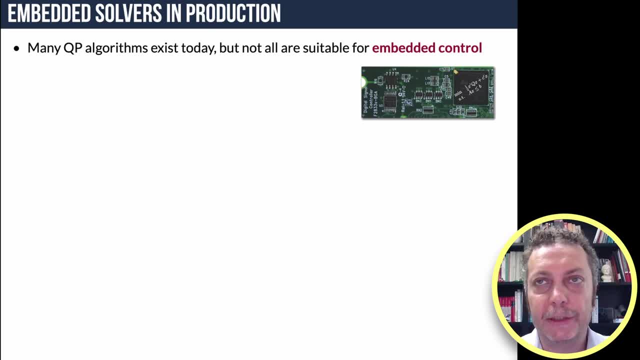 QP solution methods exist, at least from the mid-50s. As a result, many QP algorithms exist, are available in the literature, also in the public domain and also in commercial code. Not all of them are suitable for embedded control. 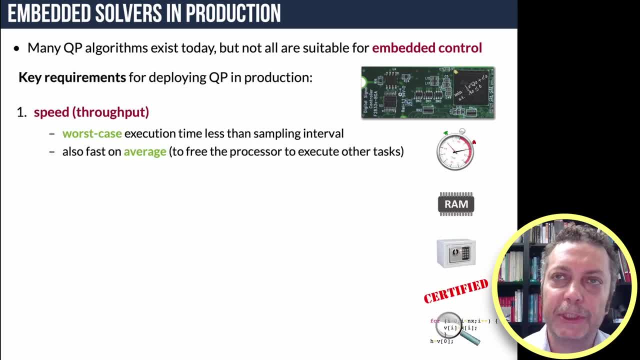 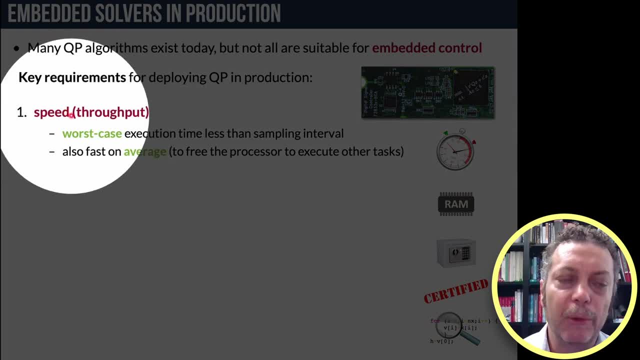 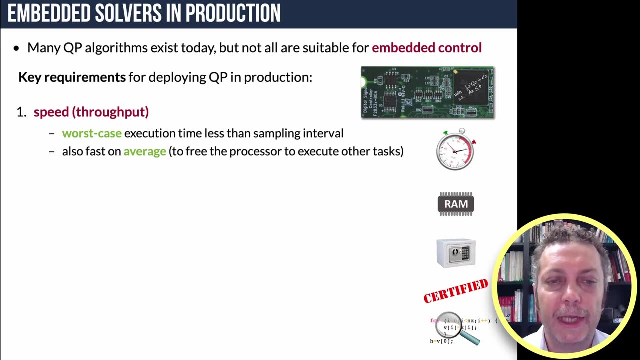 However, there are certain requirements that you need to satisfy, And I'm listing here the main requirements. First requirement is speed. So you want the solution to be computed fast enough, at least within the sampling interval, and not only on average, but also in the worst case. 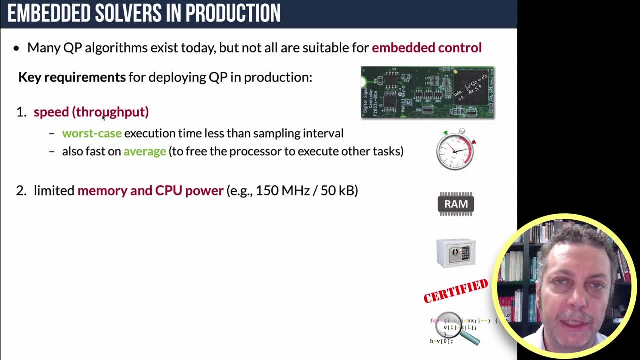 Then the QP algorithm should not require excessive memory And the throughput. so still often you are limited by the CPU power you have available and the memory you have allocated for numerical solver and for the control algorithm in general. These solvers should be numerical robust. 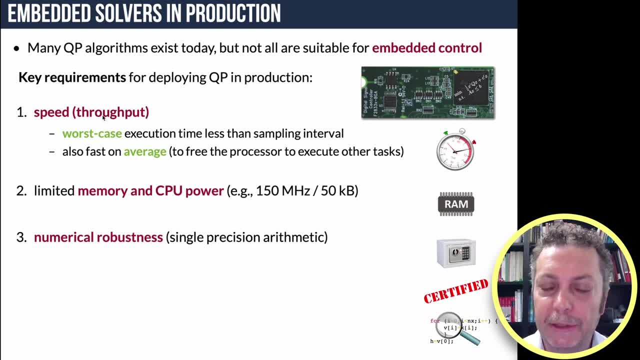 Often these algorithms are still run in single precision arithmetic. And, last but not least, the code implementing the algorithm should not be too complicated, So it should be simple. So it should be simple enough so it can be analyzed by software specialists, So it should not rely, for example, on complex external libraries. 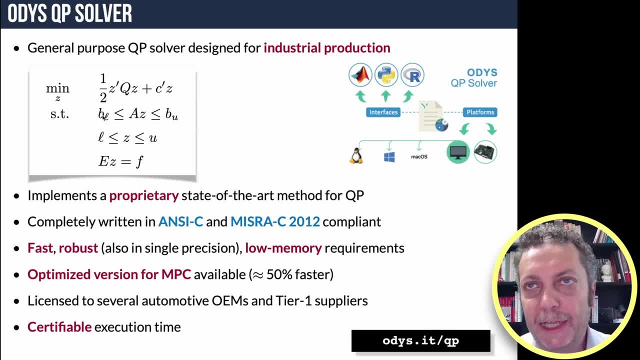 It should actually be library-free. There are many algorithms that I was mentioning. One algorithm for industrial production applications is ODIsQP, which is a general-purpose QP solution method and is written to satisfy exactly the requirements I was mentioning in the previous slide. 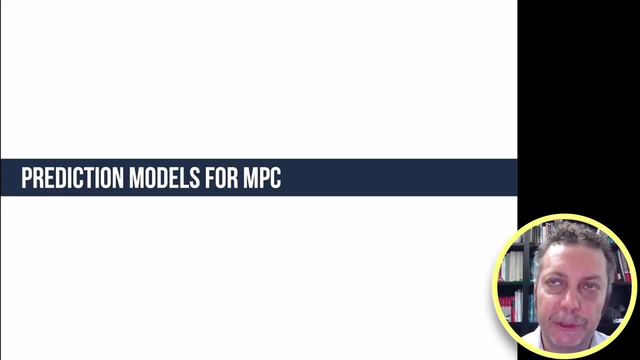 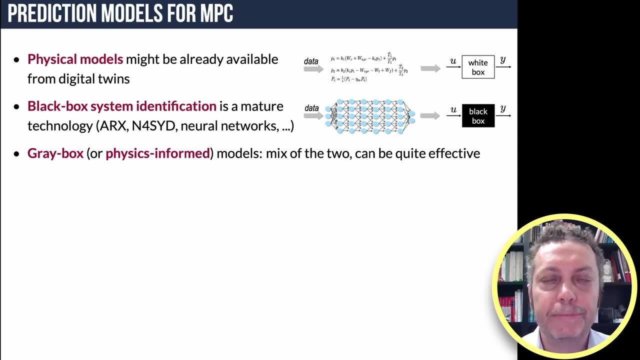 All right, now let's come to the prediction models. We need a prediction model for designing the controller Now. there are several ways of getting a prediction model. First of all, a physical model might be already available, or you can take a fully data-driven path by collecting data, experimental data. 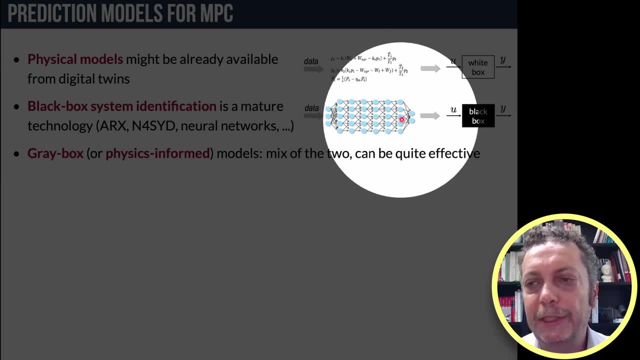 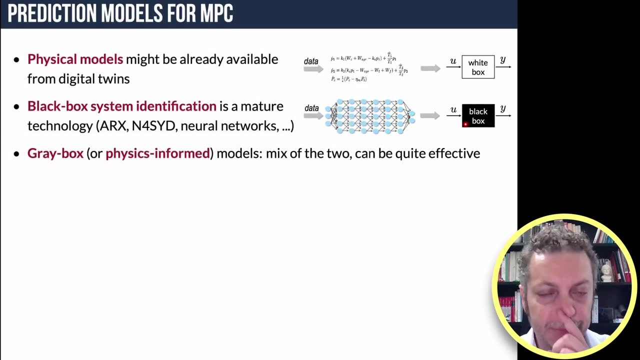 and using system identification or machine learning to get a black box model. So to understand the dynamic input output, you need to understand the dynamic input output relations of the process. Or you can have something in between, which is a gray box model where some of the model is modeled with physics and some other parts. 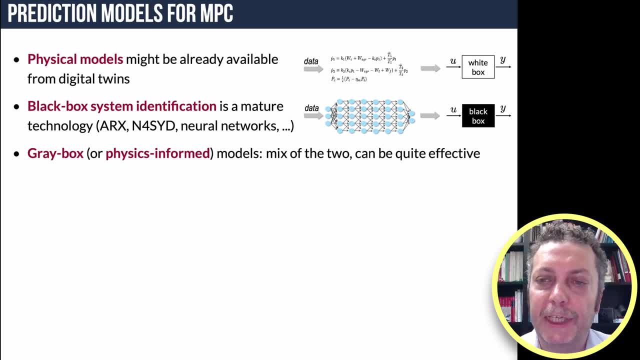 that you don't know how to model or you don't want to model in detail, can be captured by black box models. Now should the model be perfect? Well, actually no, We have to remind. I like to cite this saying by the famous statistician: 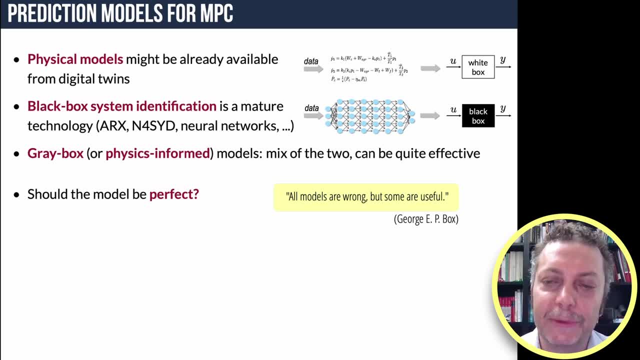 the famous statistician of the black box. All models are wrong, but some are useful. So we just need to find the model that, even if we know it's wrong, it's useful enough for MPC design. So how can we say that the model is good for MPC? 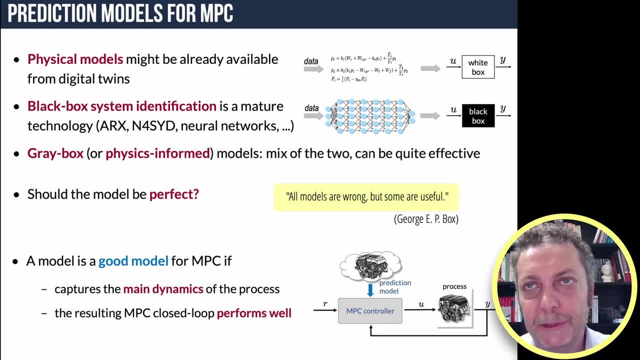 Well, it has to capture the main dynamics of the process, Otherwise the predictions are completely off and therefore the model is useless. And how can we compare different models? Which one do we want to pick? Well, usually you look how the model performs when used for MPC. 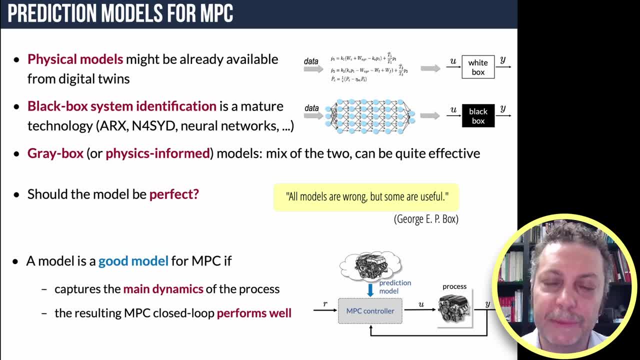 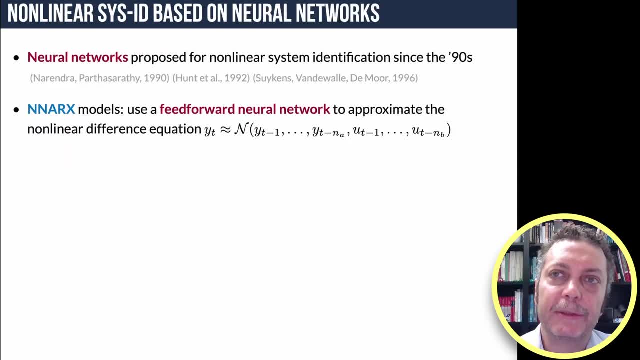 So how actually the MPC closed-loop system performance is when you use that model? Now, regarding black box models, neural networks have been quite popular to capture black box nonlinear dynamics already since the 90s. Nowadays they're even more popular. First type of model you can use: 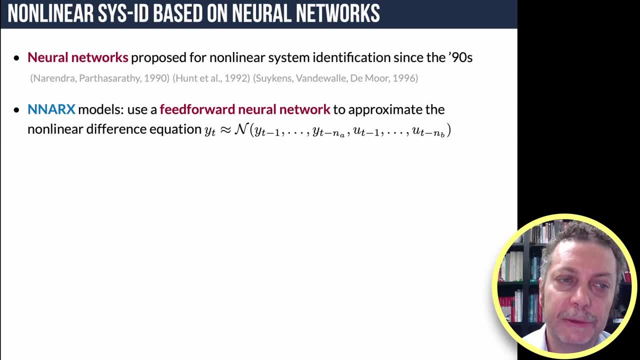 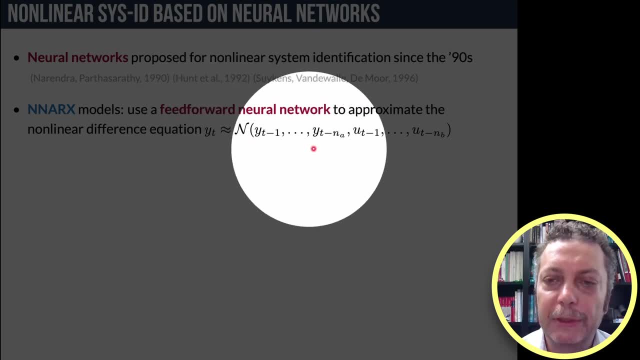 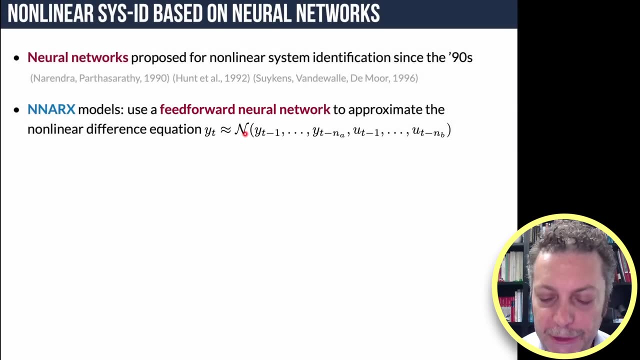 are neural autoregressive models, where the relation between the output and the previous NA values of the outputs and previous NB values of the inputs are captured by a neural network, Or you can use neural state-space models, which is even better for MPC design. 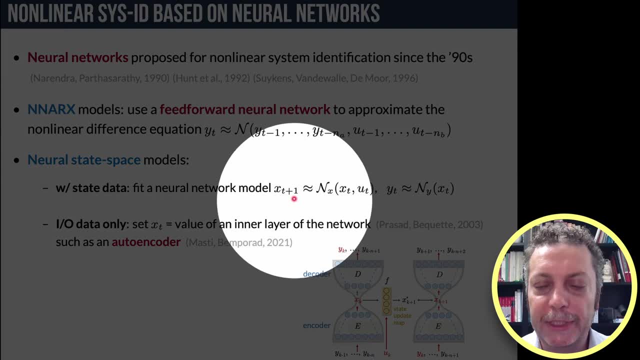 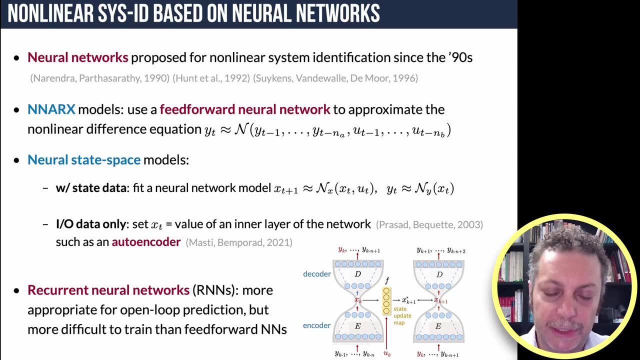 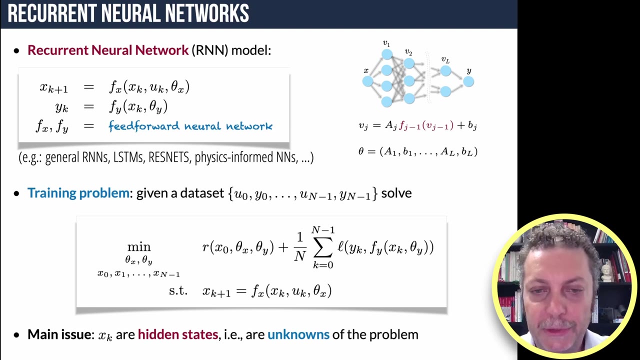 If you only have inputs and outputs available, so you don't have states predetermined, then you can use recurrent neural networks. So these are also state-space models with hidden states where structure is quite general. So say, you have a data set of a certain number of inputs and outputs. 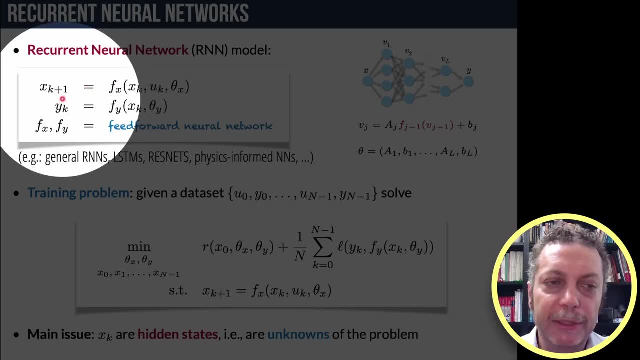 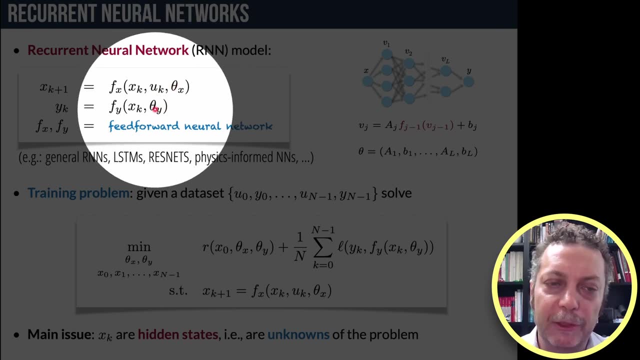 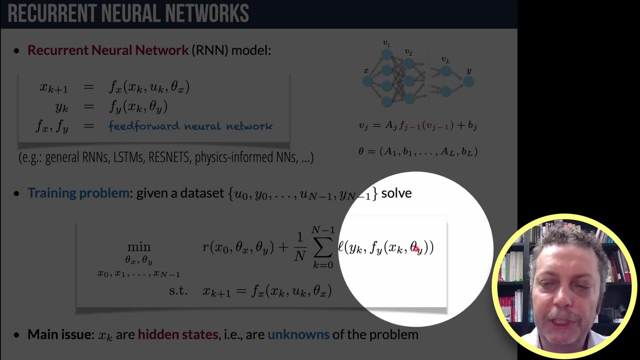 So you can try and fit a model where the state, update and the output functions are neural networks that depend respectively on some vector- theta x and theta y- of coefficients, And solve the following problem. So find the vectors of coefficients, theta x and theta y, such that the predicted outputs 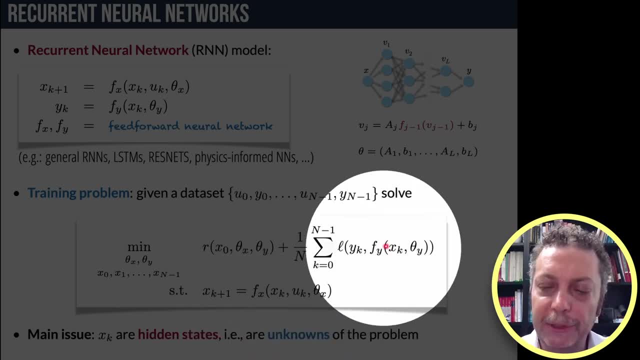 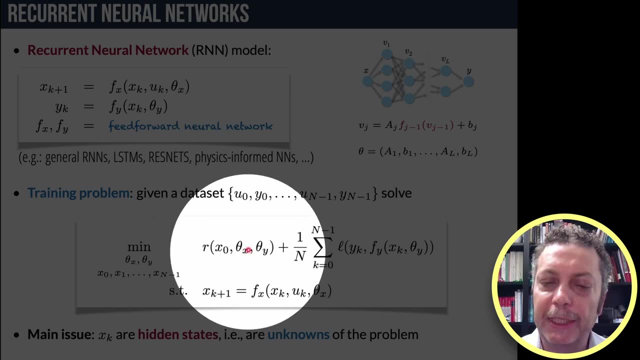 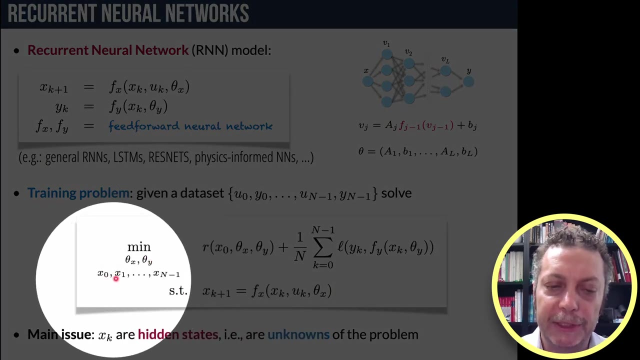 so the output that you predict in open loop by running the model match the outputs that you have in the data set, with some penalty on the initial state as well as some regularization. So the unknowns of this problem are the parameters of the network as well as the sequence of states. 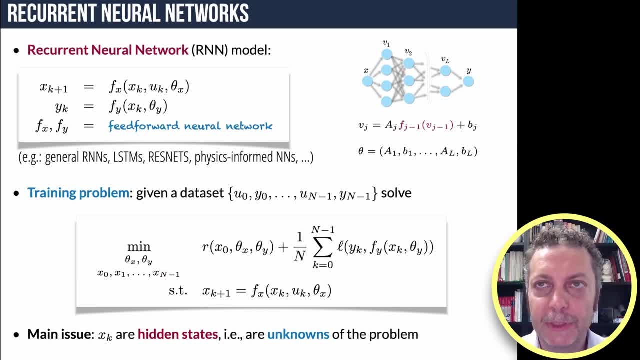 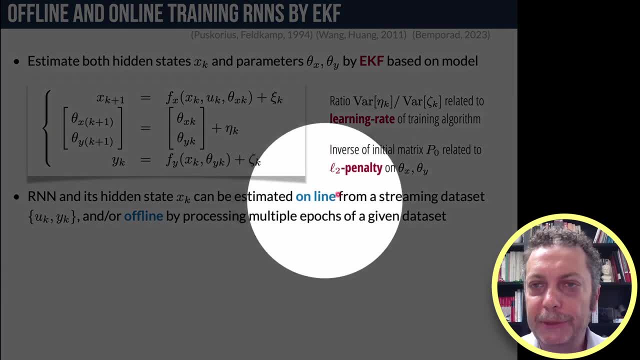 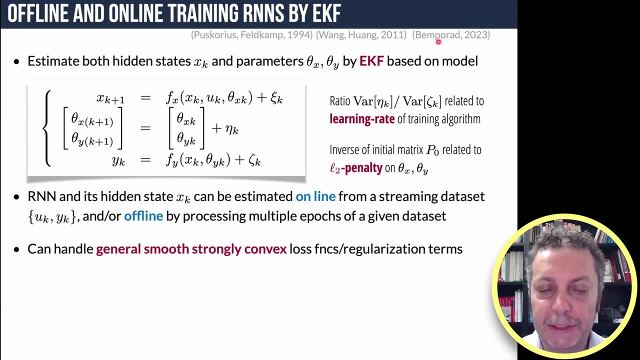 Now this problem can be solved by non-linear programming. There are a few techniques available. A technique that I have been recently investigating is to solve the problem by using extended common filtering. What I've done recently is to extend these techniques to handle arbitrary convex and smooth losses. 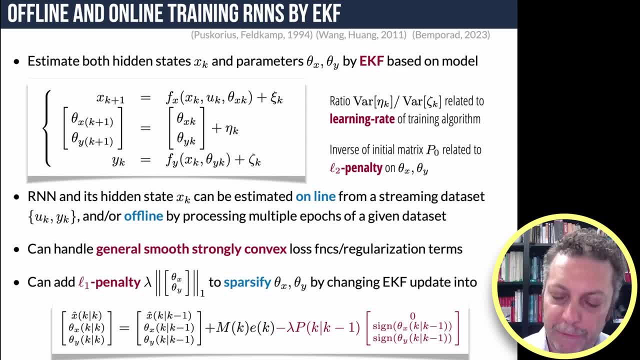 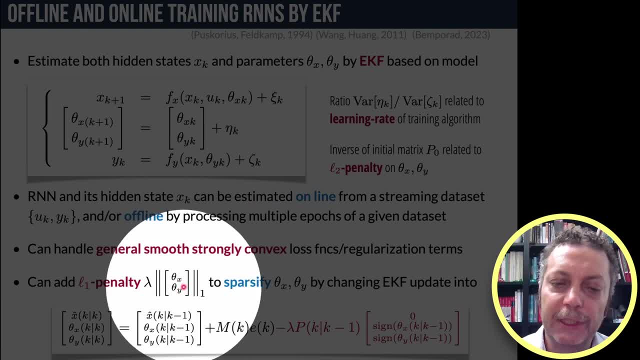 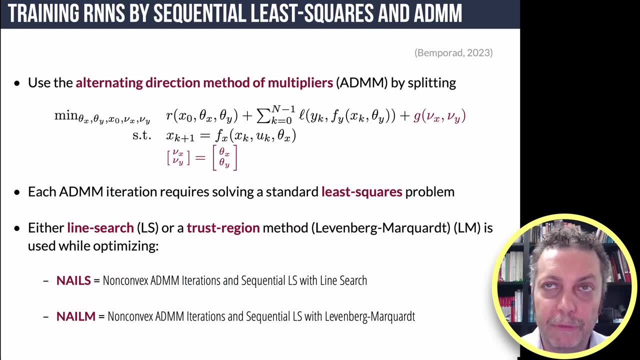 You can also handle non-smooth convex penalties, for example in the case of L1 penalty. So you penalize the one norm of the vector coefficients in order to get a sparse model And another method that I've been looking at recently for computing offline. 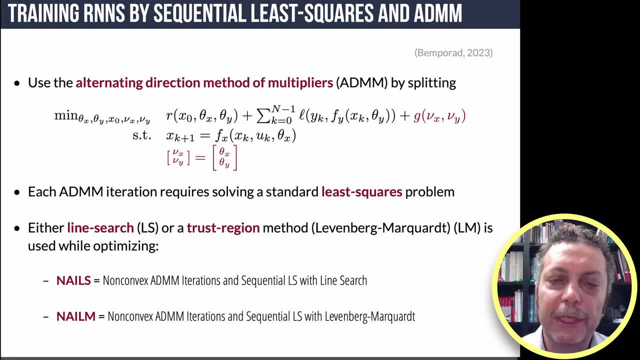 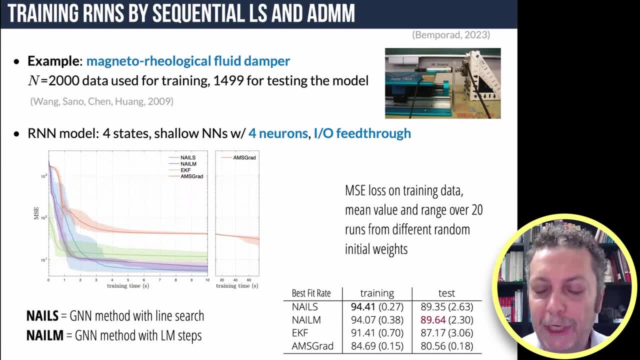 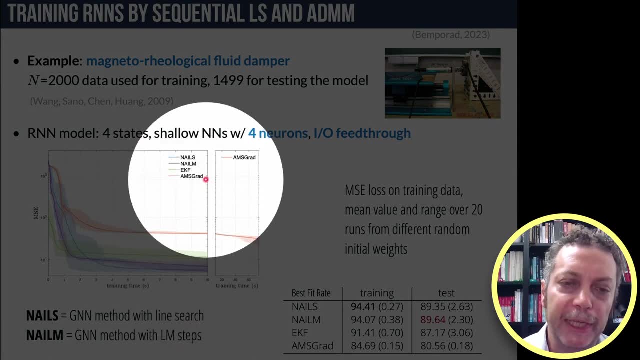 so for fitting offline recurrent neural network models is a combination of ADMM, the alternating direction method of multipliers with least squares. Let me show you an example comparing the use of this method: ADMM with least squares. So ADMM with least squares. 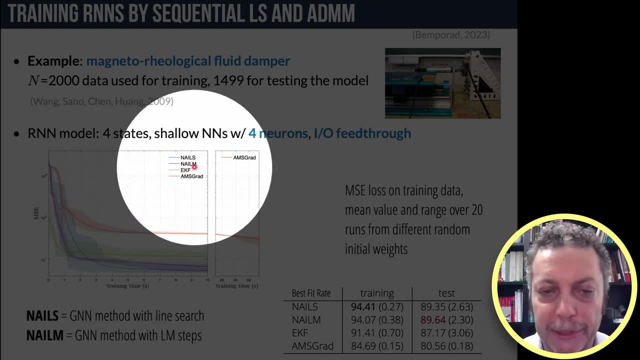 or Leveringberg-Markert, which I named NAILS or NAIL for if you use Leveringberg-Markert with EKF, and one of the most popular methods in using machine learning for recurrent neural network, which is a stochastic gradient descent method. 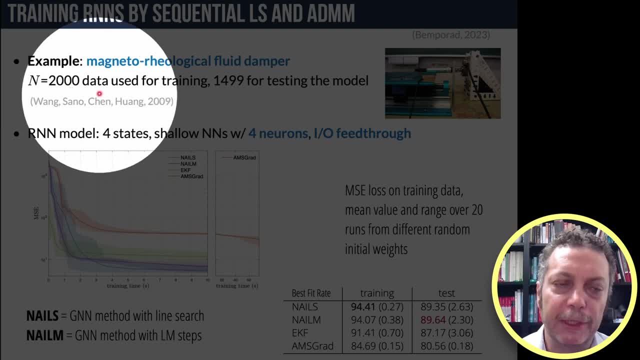 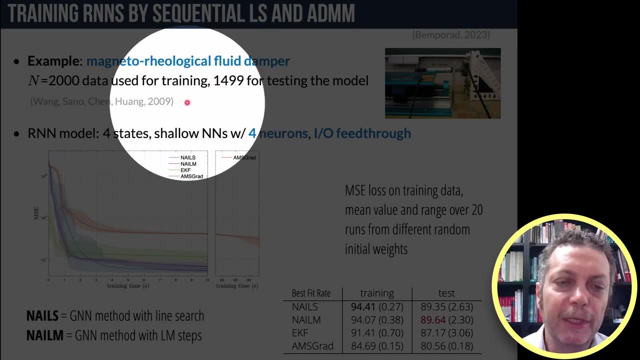 Here. the dataset consists of 2000 samples of a magnetorheological fluid damper system and about 1500 are used for testing the model. Now this is the result you get with a very simple recurrent neural network model with four states and a shallow neural network. 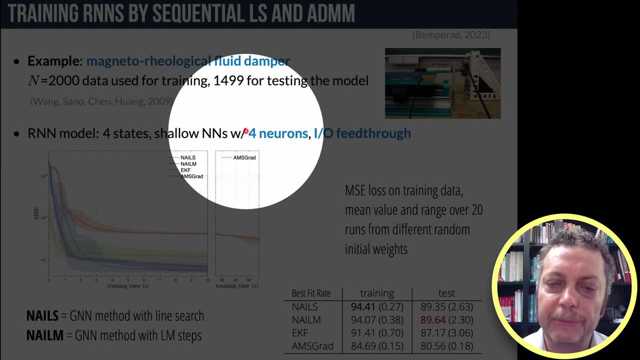 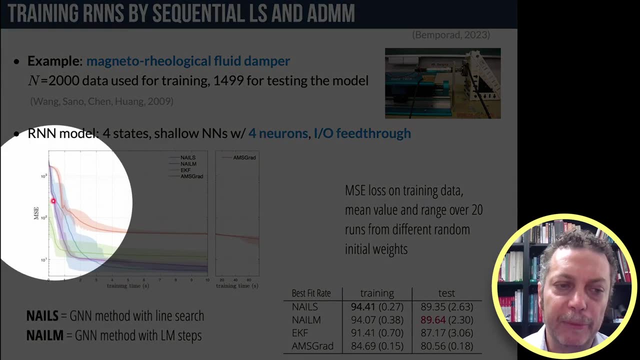 for each. the state update and the output function with four hidden neurons each. Now, as you can see here as a function of training time, this is the performance, the mean square error obtained by the model, and the one you see here in red is gradient descent. 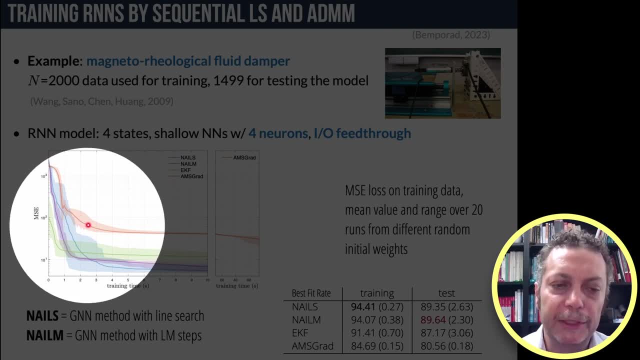 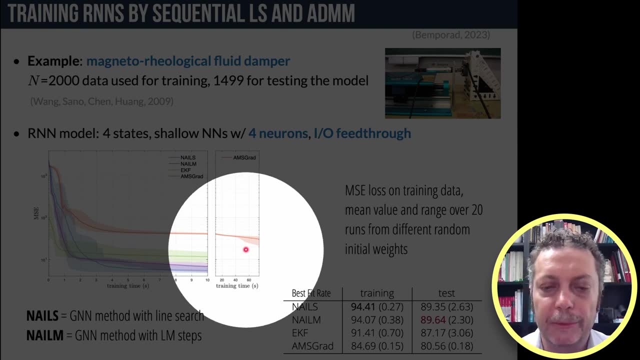 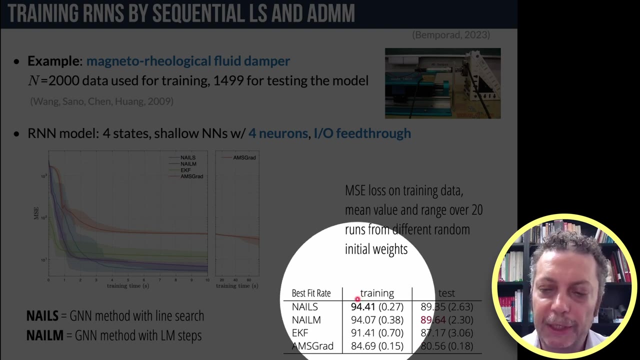 As you can see, this happens quite frequently. it's actually slower to converge where slower means you really have to wait quite some time in order to decrease the loss. So the best fit, perfect fit, is 100% and 94.4 is quite good best fit rate. 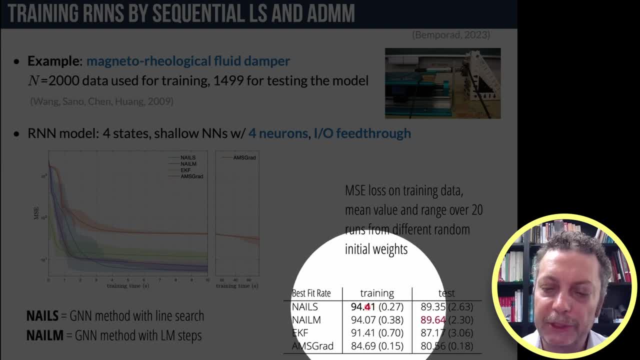 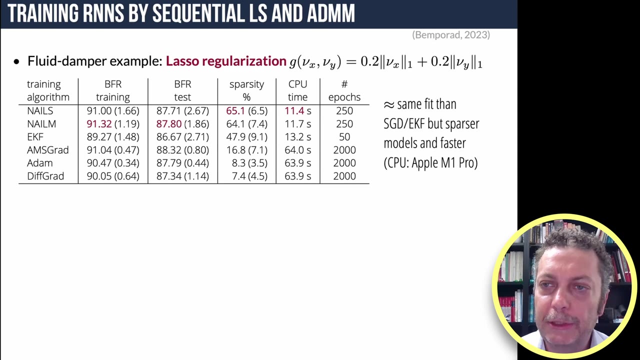 and so, in this case, NAILS performs the best on training. Actually, the version with Leveringberg-Markert gives slightly better result on test data, which is ultimately what you want to get. Now let's introduce L1 penalties. So let's say you have a penalty 0.2. 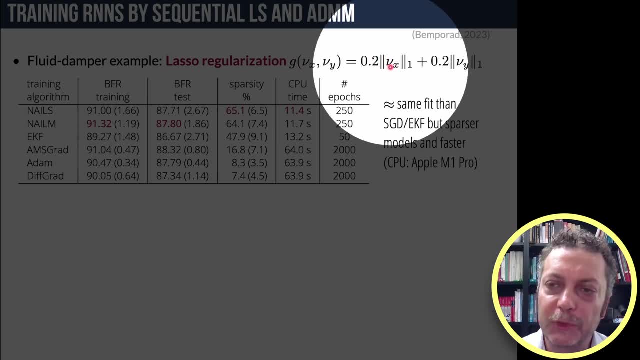 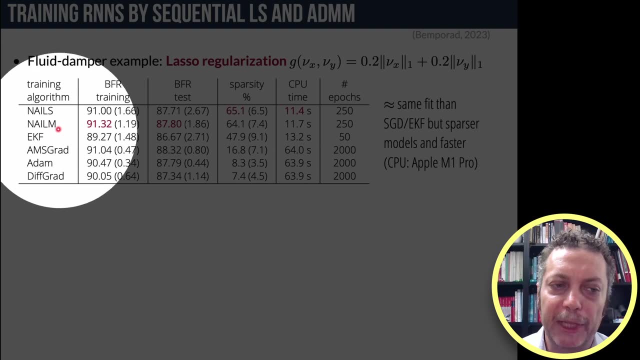 on the one norm of the coefficients of the weights and bias term of the neural network, of the state update function and the output function. Here I'm comparing again the same algorithms and three different stochastic gradient descent methods: Amsgrad, Adam and Diffgrad. 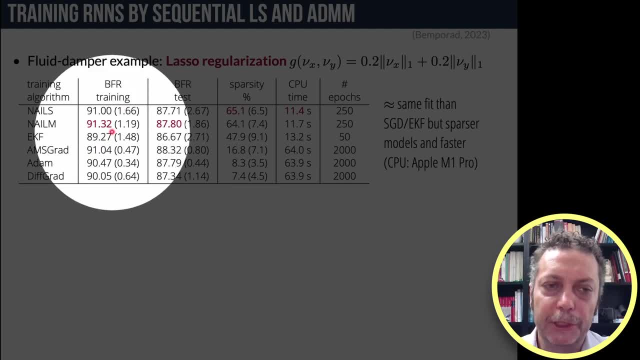 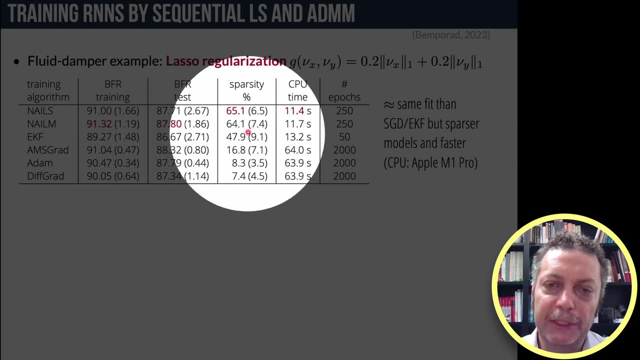 and, as you can see, they all reach more or less the same best fit rate on training data and on test data. What is interesting here is the sparsity that you get. With NAILS, NAILS and extended kernel filtering, you get quite some sparsity. 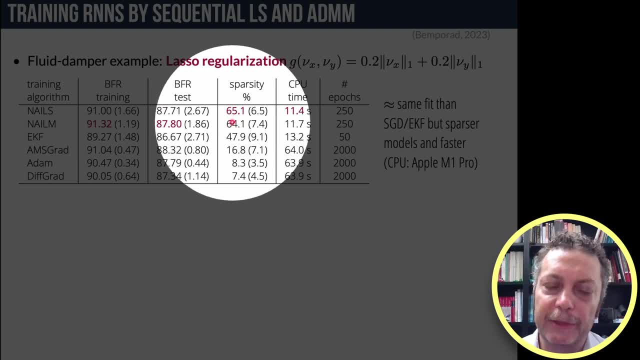 so about 65% sparsity here and 47, about 50%, say, sparsity with EKF in a computation time overall in the order of 11, 13 days, While with stochastic gradient descent methods you get similar performance. 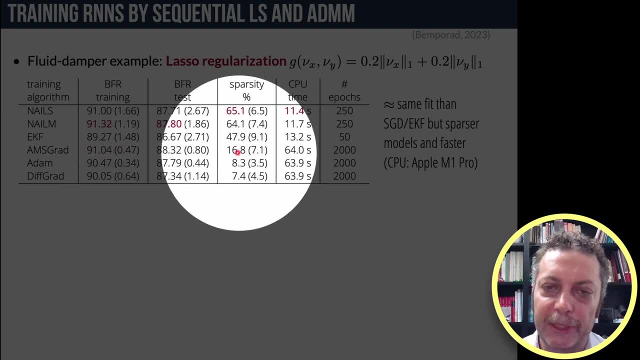 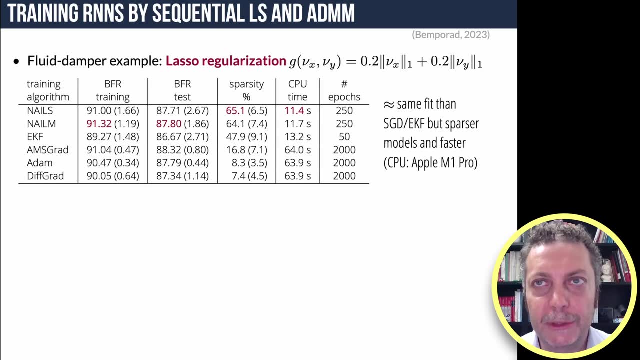 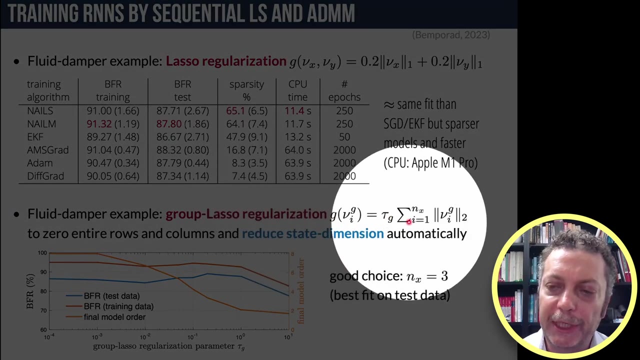 but it takes a longer time and the model sparsity is not as good as if you use these other methods that exploit sort of approximate second-order information of the cost function. And here is another example where here I'm using group loss of penalty so to try to remove states from the model. 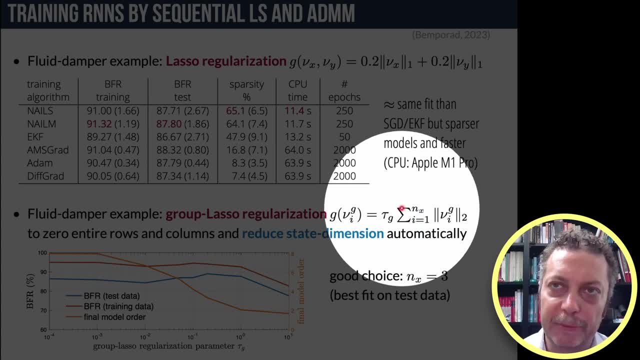 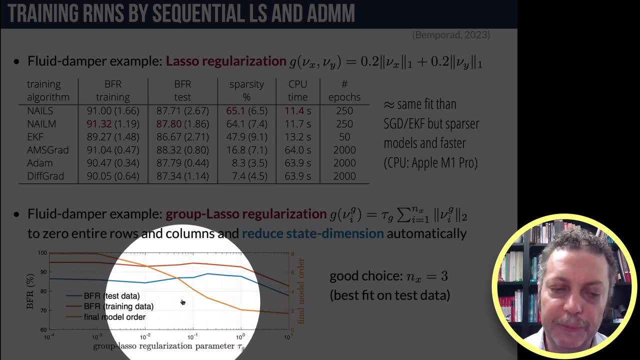 so grouping together the coefficients related to the same state And, as you can see here, as a function of the regularization parameter for the group loss. of course, if you increase the penalty a lot, then the model quality starts becoming poor. Of course the model order will diminish. 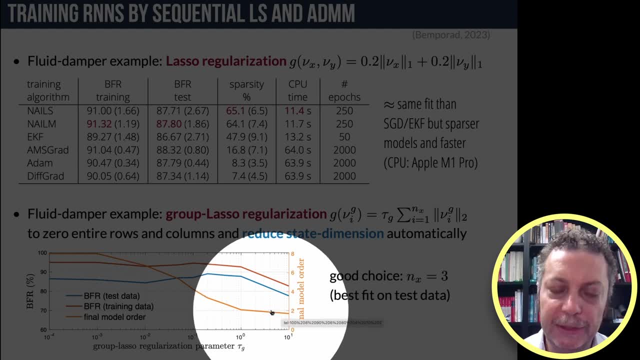 because more and more states will be redundant. But you can choose here, for example, around this point. here you have still pretty good quality of fit on training and the test data and a model order which is small. For example, here you have a model order. 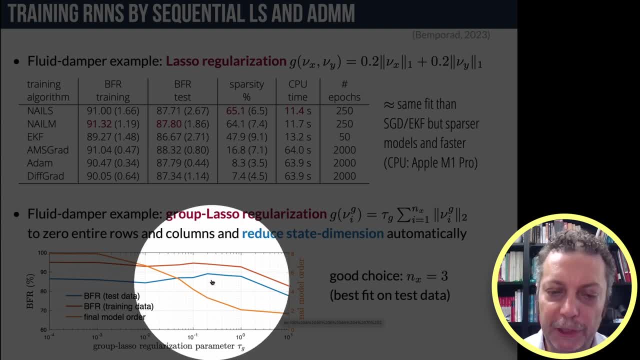 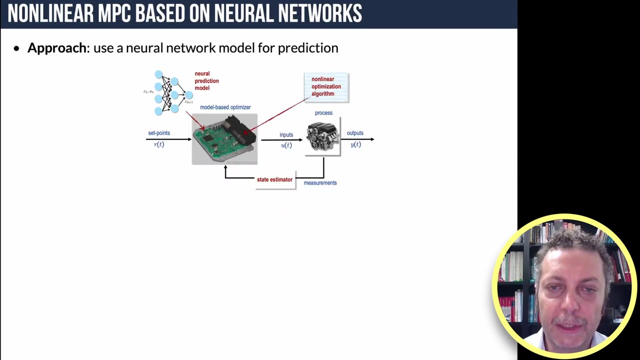 of three states, You actually get the best fit result on test data, And so this will be actually the model order you want to choose for this particular data set. So what you do now with the model? well, the idea now is to take the model. 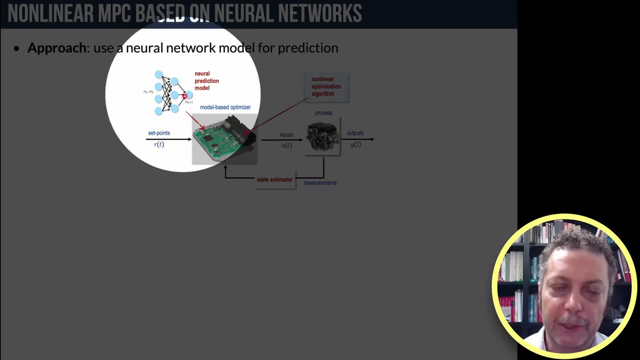 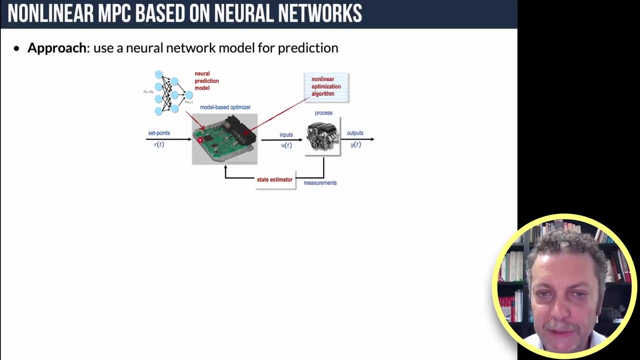 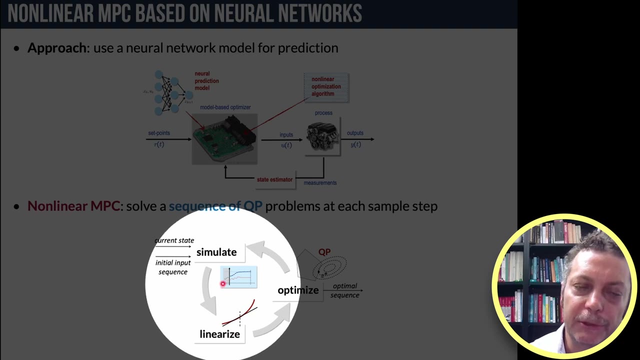 we have identified, So, for example, the recurrent neural network model, and use this directly as a prediction model for MPC. So the resulting MPC control will be nonlinear. So the way to solve the nonlinear MPC problem, one way of solving the nonlinear MPC problem, 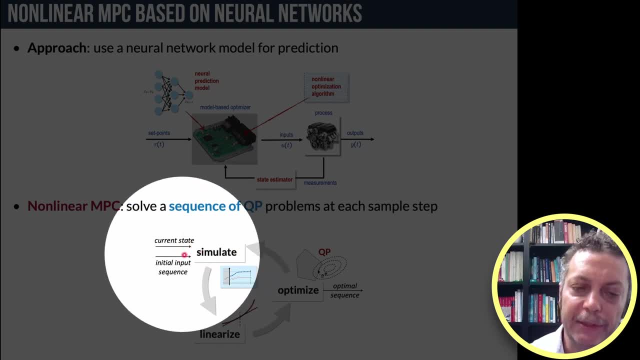 is given the current state and an initial guess for the input state. For example, it could be the previous, the remaining part of the sequence that was computed at the previous time step. You can simulate this case, the recurrent neural network model, over the prediction horizon. 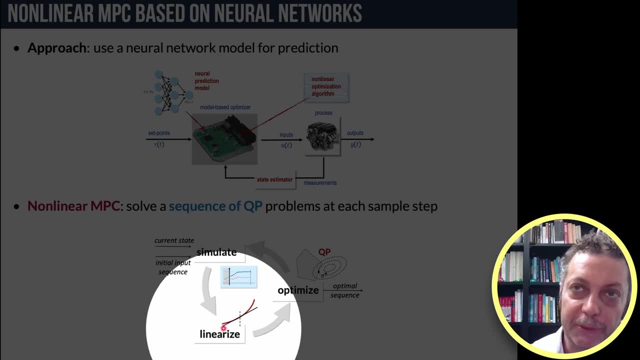 linearize the model, So get the Jacobians of the model with respect to the state and inputs and build a quadratic programming problem based on this generalization that you can solve by quadratic programming, And this will give you an optimal sequence of inputs. Now 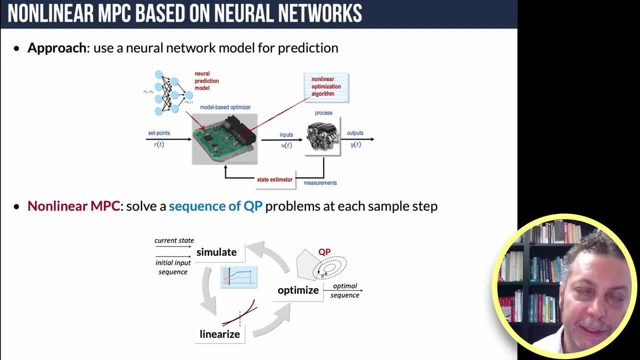 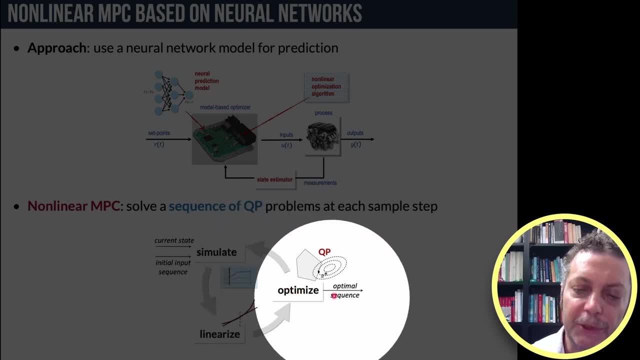 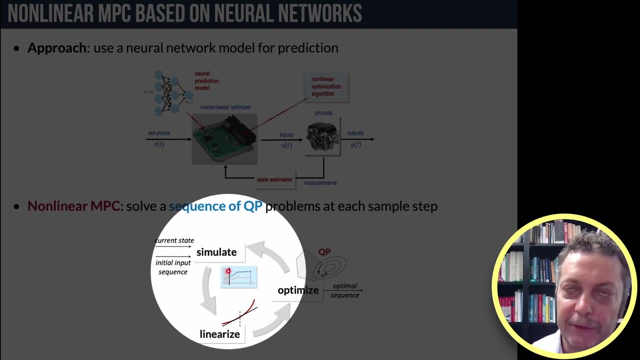 if you apply directly the first sample, you will do linear MPC. The idea here is that instead of applying directly, if you have enough computation time, you can now use the new optimal sequence to simulate again the system from the same initial state, but with a different excitation. 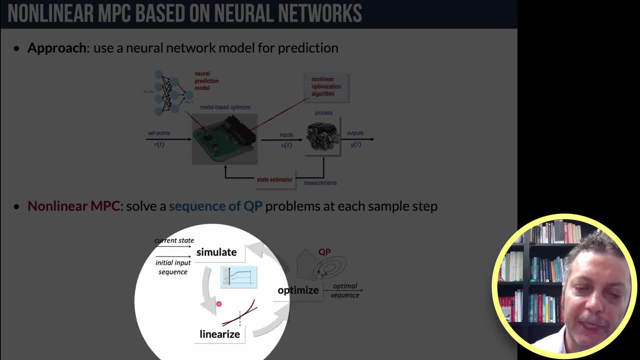 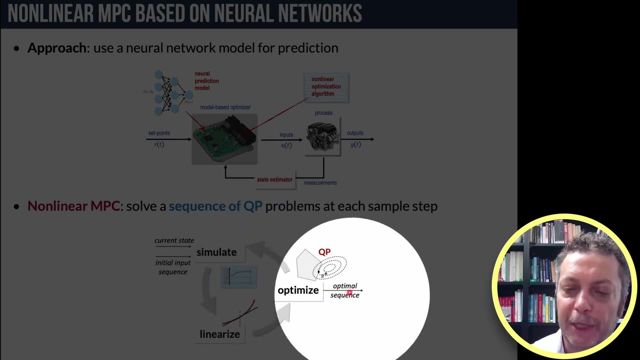 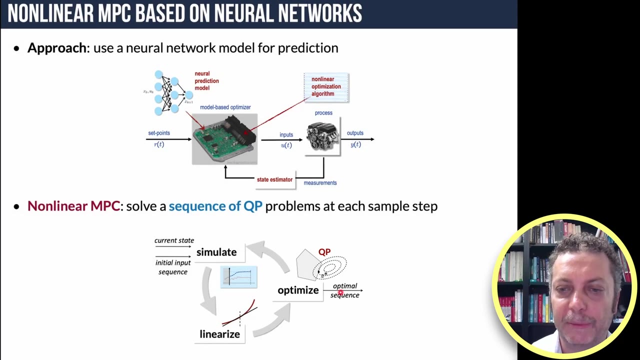 get the new linearization, solve the new optimization problem and so on, And you can guarantee convergence of this scheme if you do a line search. So, instead of directly applying the new optimal sequence, you select a sequence in between the current one and the new one that you have optimized. 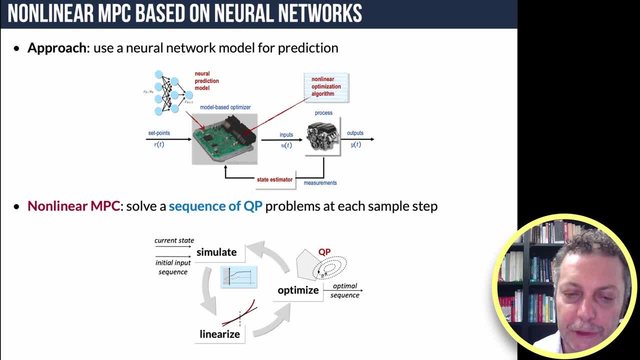 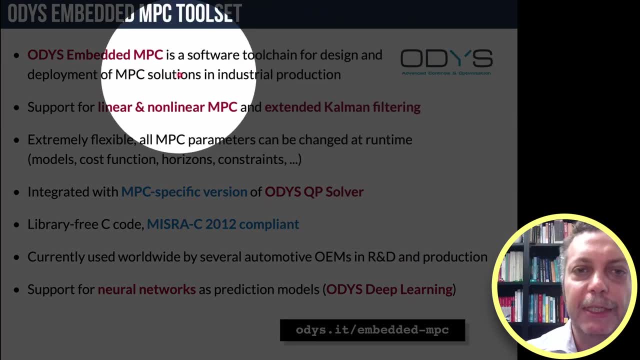 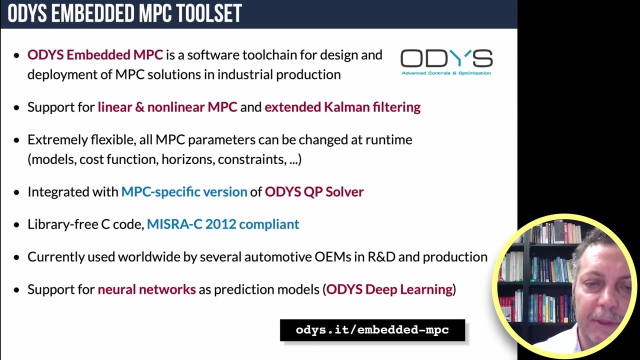 So all this approach, so this entire approach of sequential quadratic programming and non-linear MPC- this, implemented in the all these embedded MPC, which implements all the ideas that I have described and is coded in C, is actually MISRA C 2012 compliance. 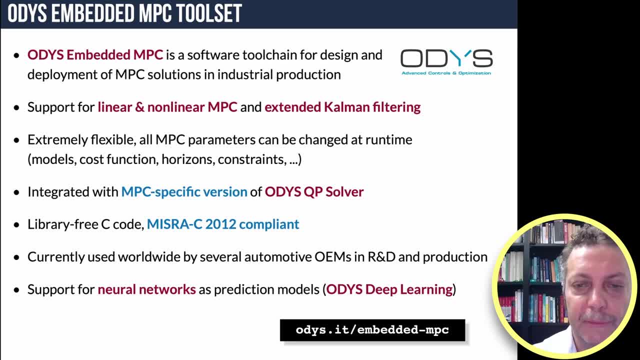 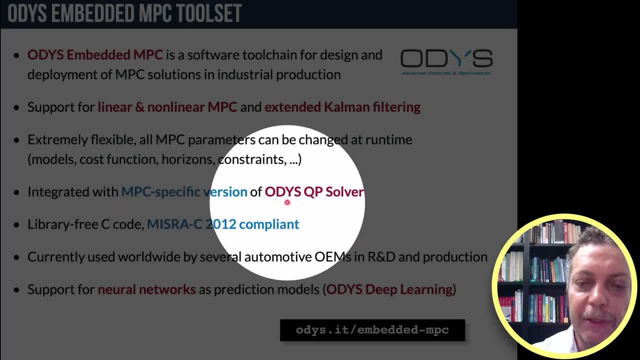 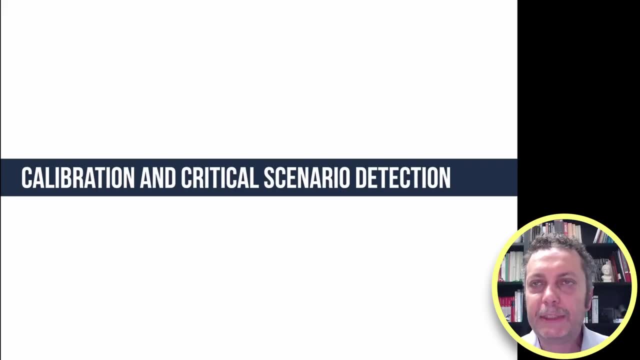 So it can be used for. it's actually used for production power positions And is using the efficient MPC specific version of the Aldous QP solver for solving the QPs that arise from the constructions. All right, now let's talk about calibration aspects. 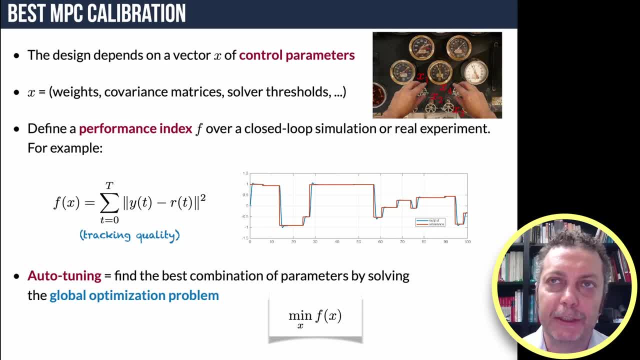 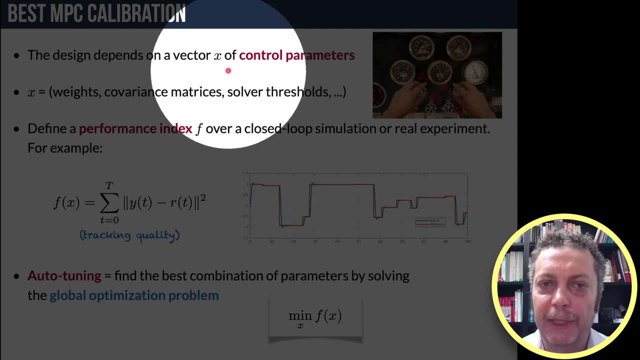 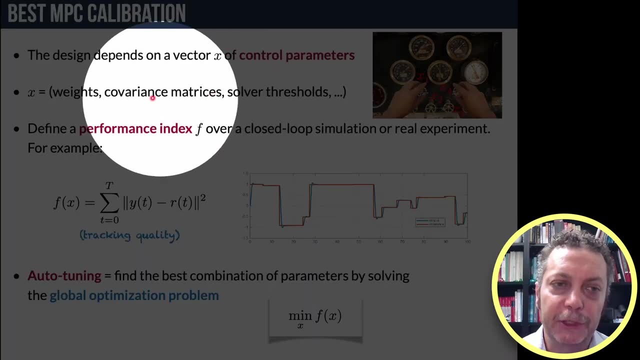 So what is the best calibration of MPC you can make? Well, the calibration depends on different parameters of the controller. So let's call X, the vector collecting all the parameters You can tune. These parameters usually are actually the weights that you need to tune. 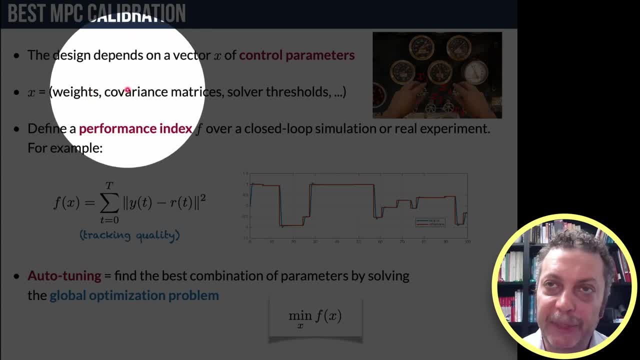 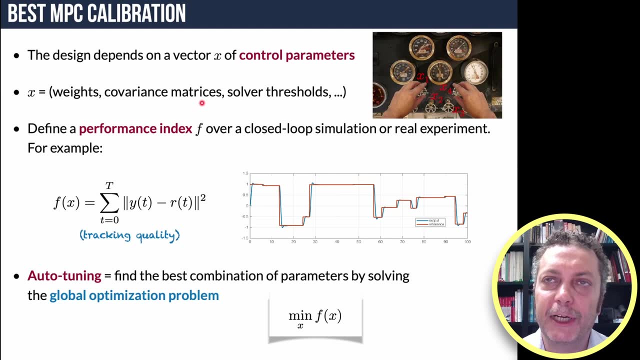 that you use in the performance index, The covariance matrices that you use in the Kalman filter, extend the Kalman filter, Then even the thresholds you use in the solver. These are all parameters that you need to tune. So how, what is the best tuning? 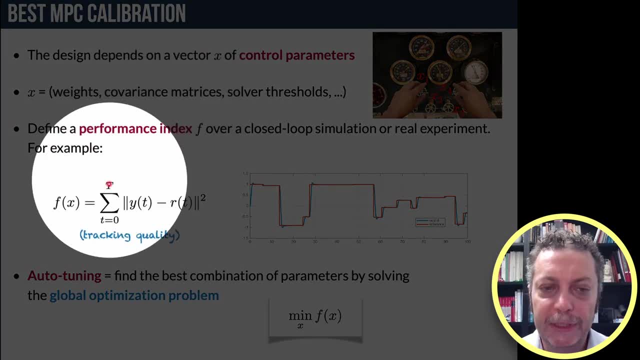 Well, if you're able to define a performance index- So, for example, this could be the sum over a certain experiment or simulation of the difference between the output and the reference you want to track- Then you can look at the problem of minimizing this function. 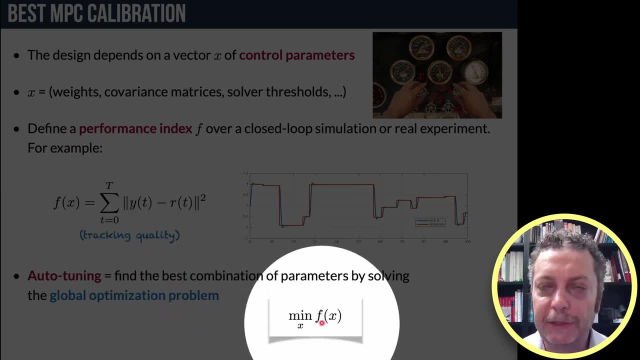 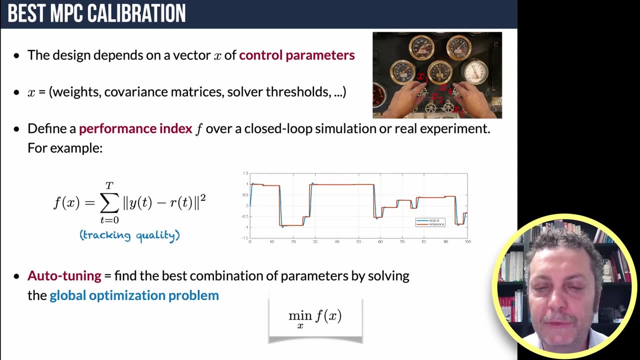 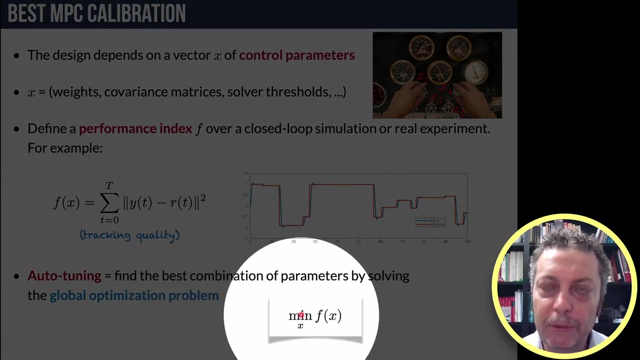 as a global optimization problem. So minimize this function with respect to X So very abstract way. If the function F captures what you want to achieve, you can use global optimization algorithms whose goal is trying to get the minimum with least number of function evaluations. 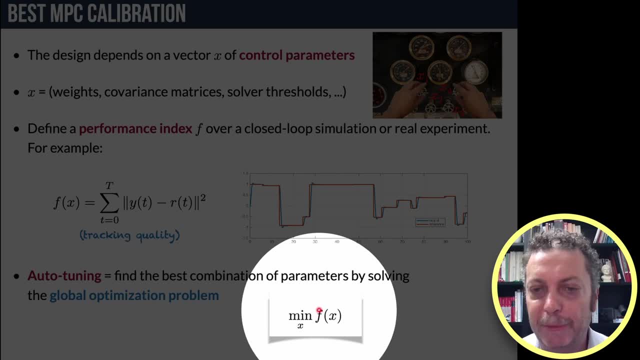 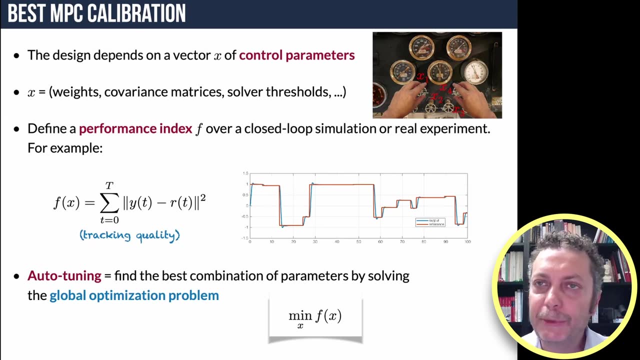 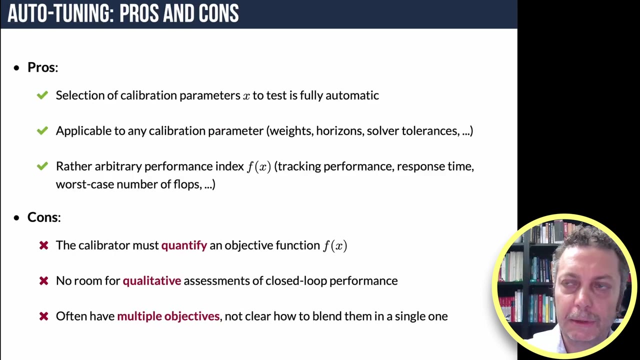 So that you can minimize the number of simulations or even experiments that you need to make. This is a totally automatic tuning of the controller And actually we have used this also in many problems. It's quite, it's quite useful. So the approach has several advantages. 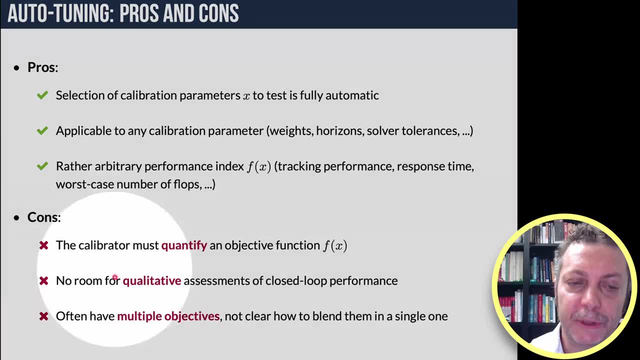 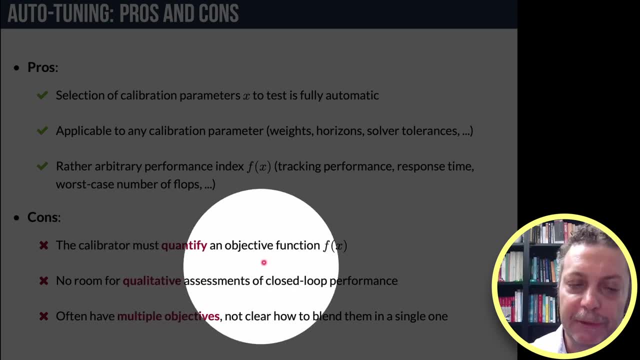 However, there are some limitations in this approach. First of all, you need to quantify an objective function. Also, there is no room for qualitative assessment, So everything needs to be quantified, And sometimes that's the reason why the function may be difficult. 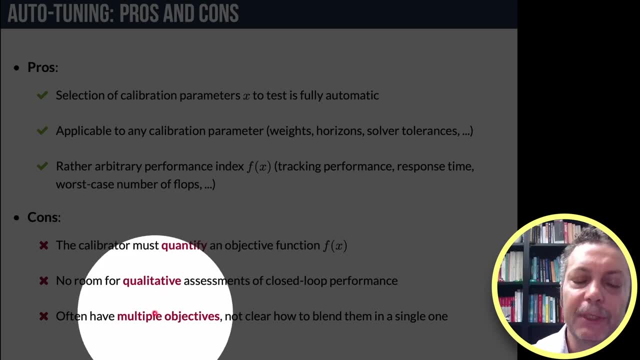 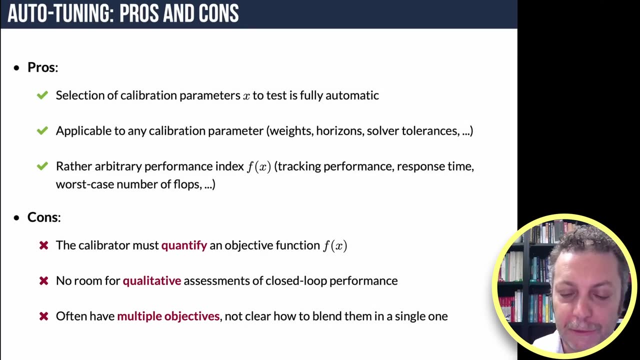 to quantify is that you have multiple objectives, So multiple objectives you want to minimize and it's not clear how you want to blend those objectives into a single function, F of X. So for this reason we have developed an approach based on active preference learning. 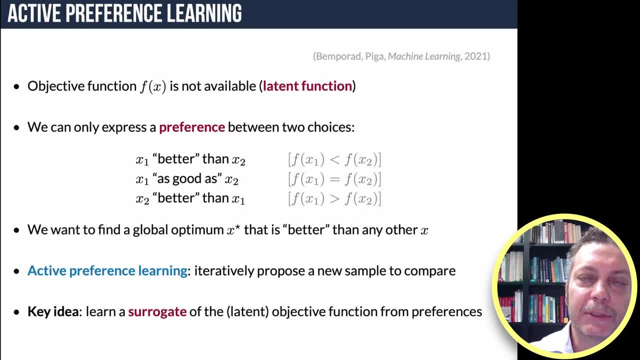 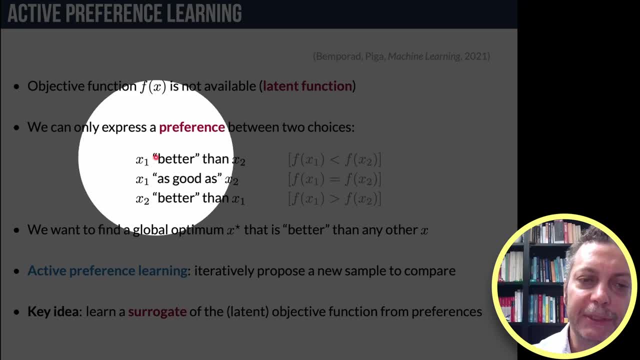 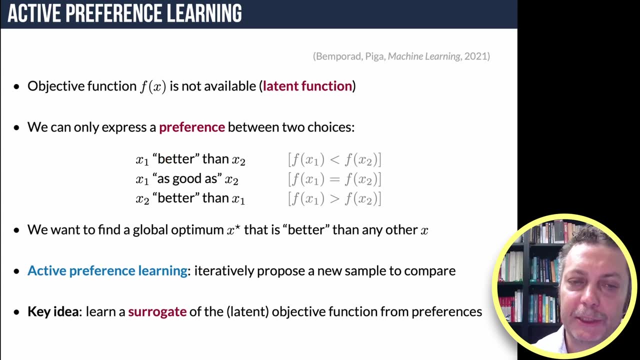 So we assume that there is no function F of X. The only information that you have is whether a certain combination of calibration parameters is better or worse than another combination. So what is actually asked to the calibrators is to say whether calibration X1 is better. 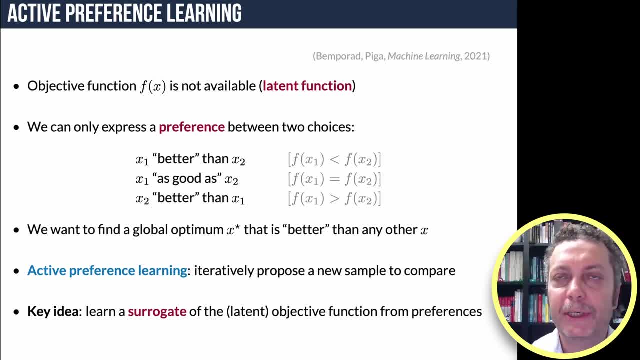 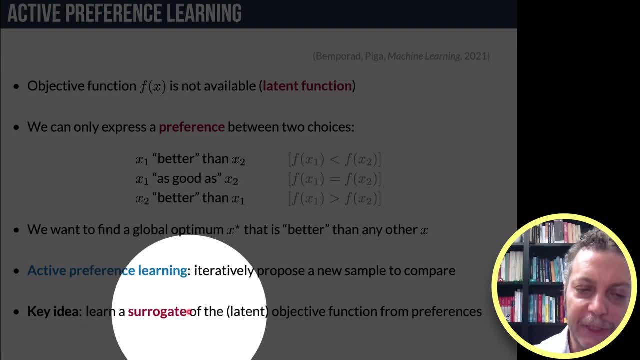 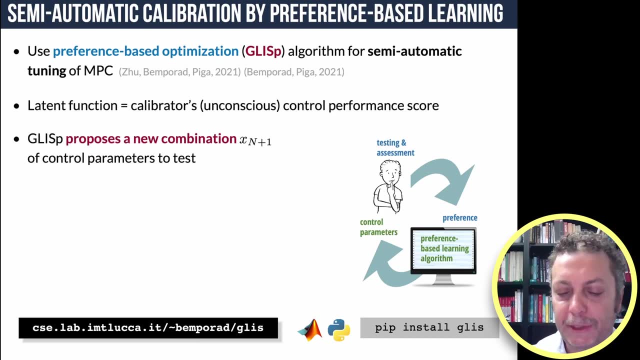 than calibration. X2 or X2 is better than X1, or they are equivalent, And so the idea is to learn a surrogate of the latent objective. We have tested this approach for semi-automatic calibration of MPC, The algorithm that we call GLISP for global optimization. 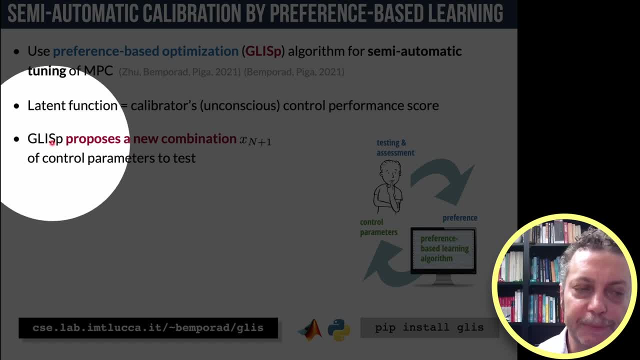 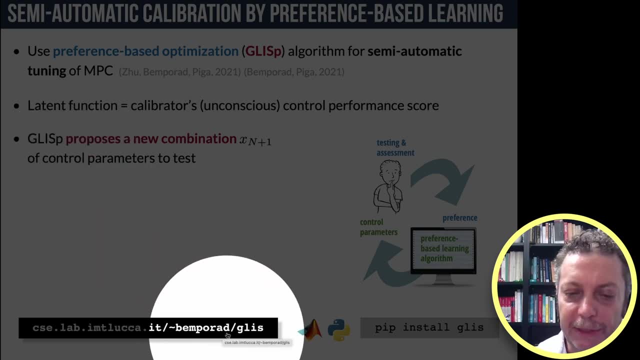 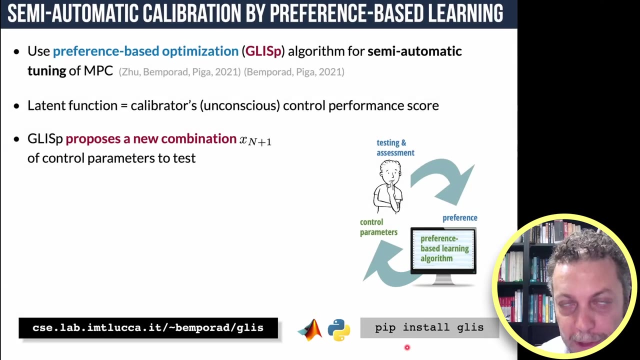 using inverse distance weighting and rather basis functions. P is for preference based. Actually, this algorithm is part of the package that is really available. You can use it in Python with pip install. It implements both the global optimizer and the preference based global optimizer. 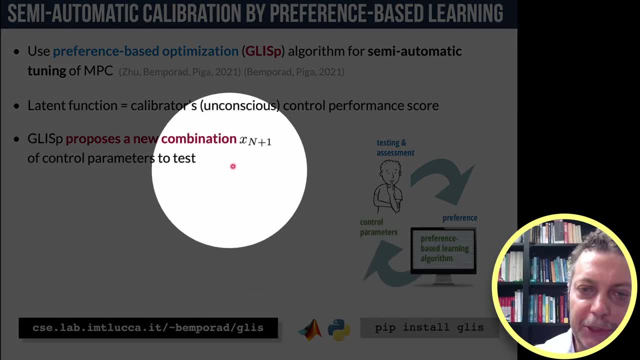 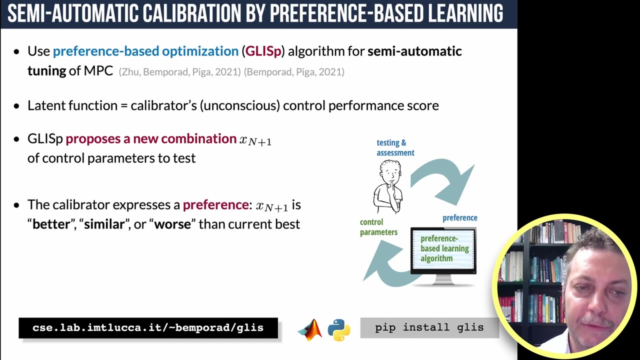 So the algorithm proposes a new experiment or simulation to run to the calibrator, which will execute it and will tell whether the new combination is better or worse, or the same. that's, then, the current best found so far, And this algorithm, this amazing piece of information. 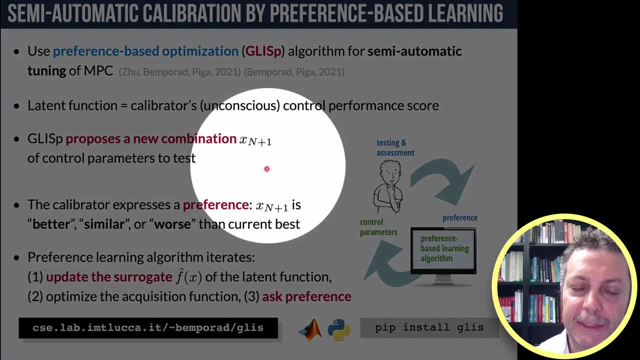 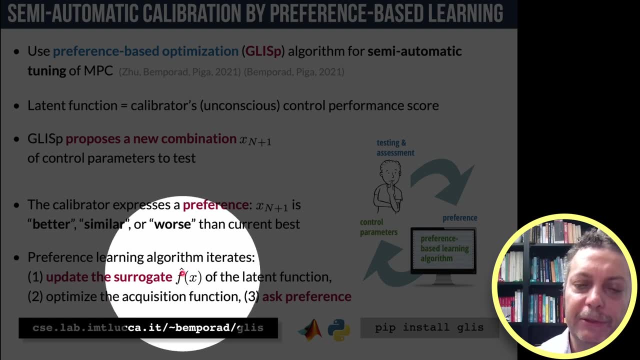 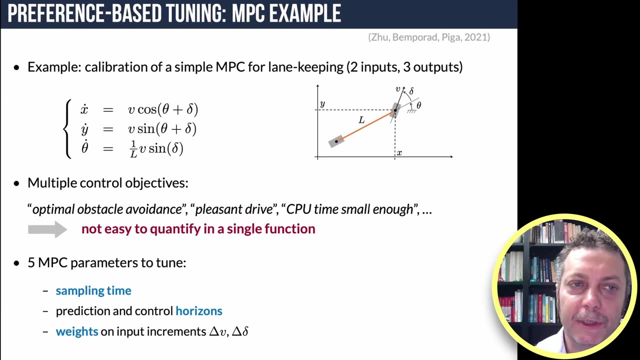 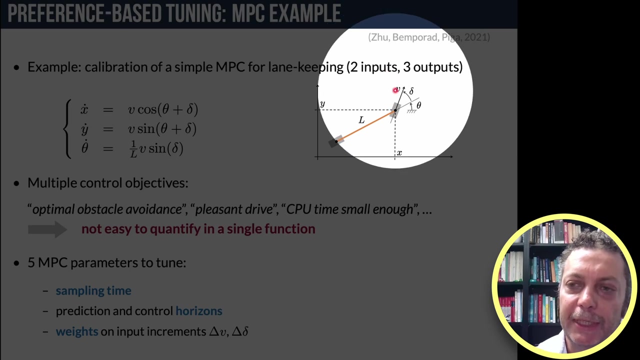 the preference is based to update the surrogate and by minimizing the combination of the surrogate function and an exploration function, the algorithm will propose another combination to test and so on. And here is an example: This is an MPC for lane keeping two inputs: velocity and steering angle. 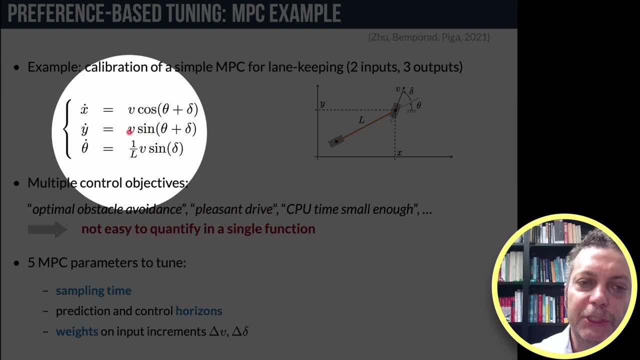 and three outputs. So now, what you want to achieve, which are your objectives? Here you have multiple objectives. You want to have optimal obstacle avoidance. You want to avoid hitting obstacles. You want to avoid obstacles in an optimal way. You want the drive to be pleasant. 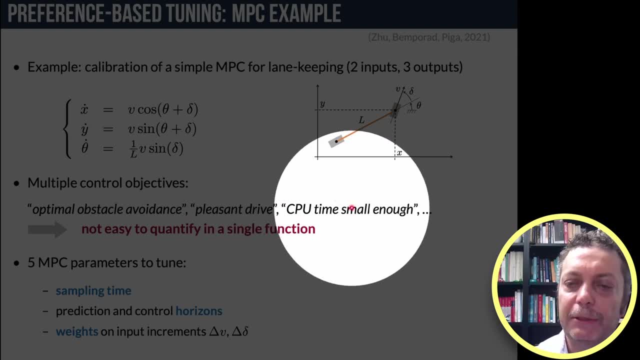 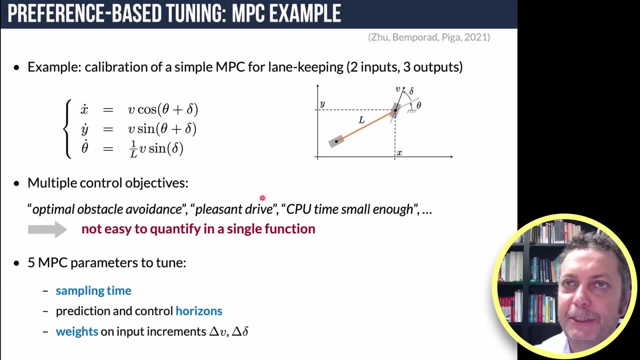 for the passengers And you want the controller that is not too much expensive from the computational viewpoint. So these three objectives in particular are not easy to quantify in a single function, And what we need to calibrate here are five parameters which are: sampling time, 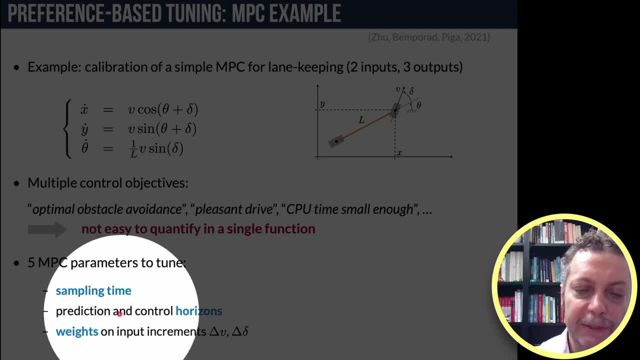 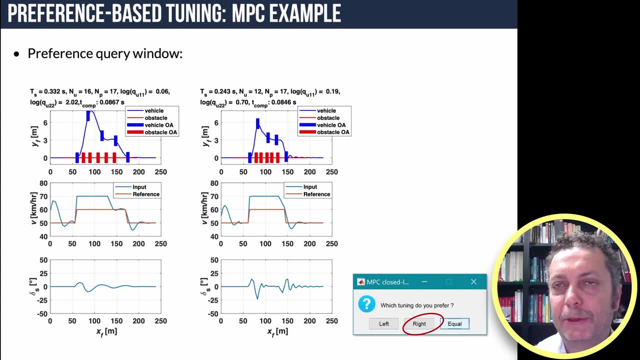 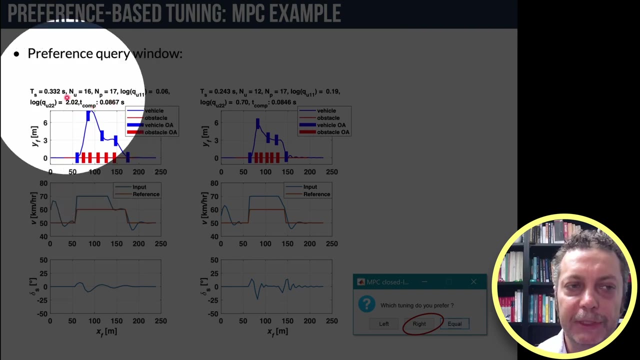 the controller, the prediction and control horizons, as well as the weights on the input increments. So here's a snapshot of the algorithm running. So the algorithm will propose two combinations of sampling time and horizons, And in this case we optimize the logarithm. 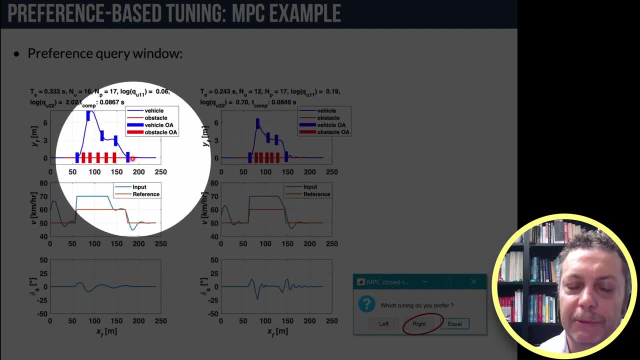 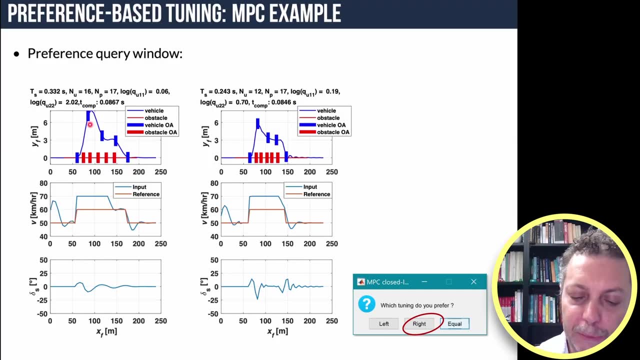 of the horizon. So in this case, the algorithm will choose one of the weights and then you decide which one you like the most. So in this case we prefer the one on the right. Click right, And these run multiple times At the end. 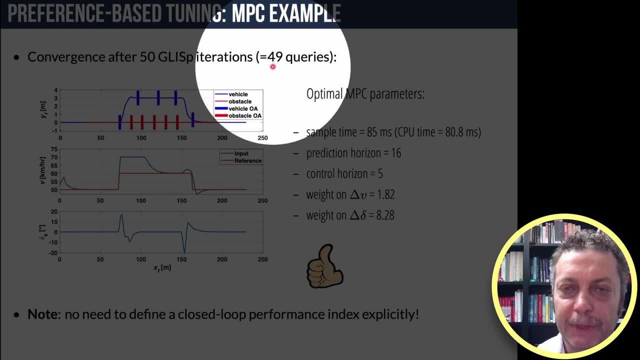 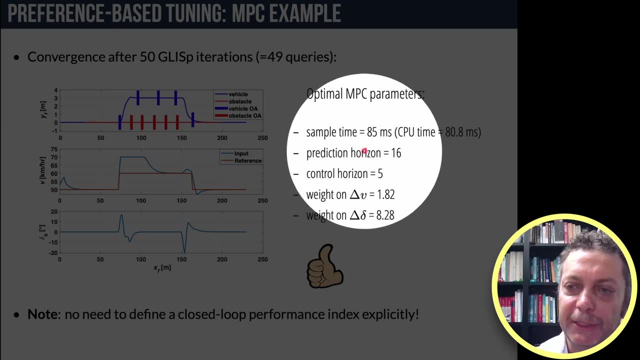 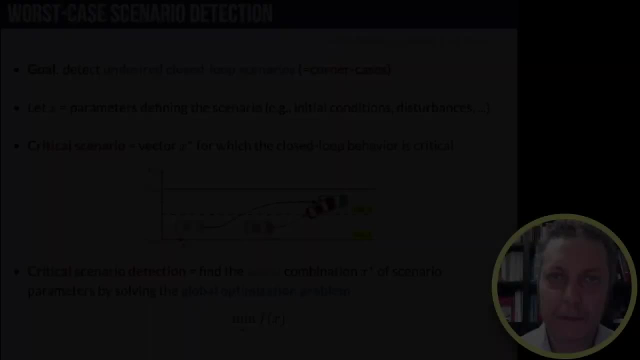 after 50 iterations, which means after asking 49 queries, the algorithm will converge to a design. in this case, sample time of 85 milliseconds, prediction horizon 16, and these two weights on the input increments. So let me finally mention 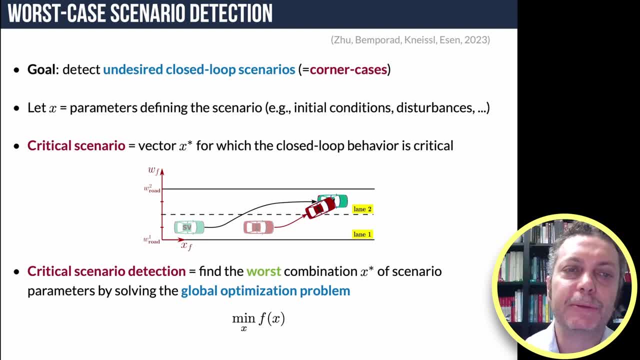 another application of global optimization. So using the same least algorithm I was mentioning before for globally optimizing performance, Here we use the global optimizer for the opposite problem of finding the worst case, So the worst performance we can get, And this is particularly useful for detecting corner cases. 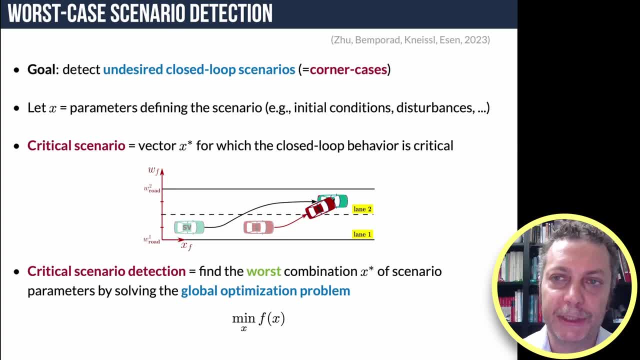 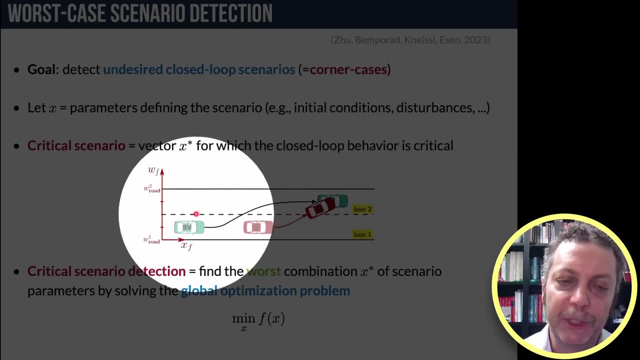 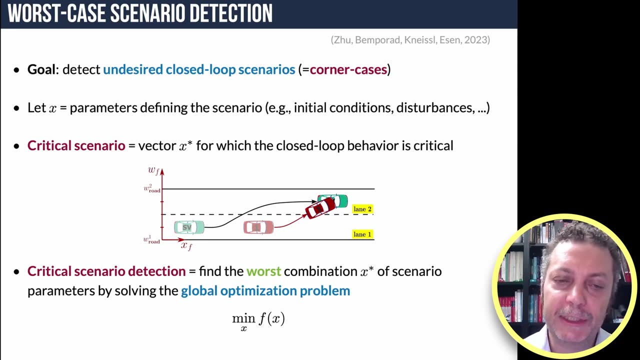 or worst case situations that we may encounter. This is a work we did recently where we looked at, in particular, at the problem where we have actually the same controller and PC controller that was described in the previous slide used now in simulation. You want to make sure. 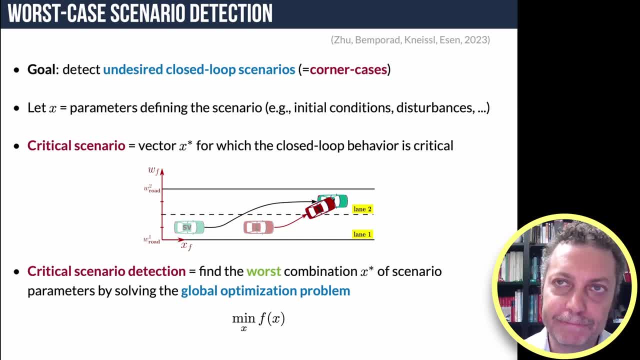 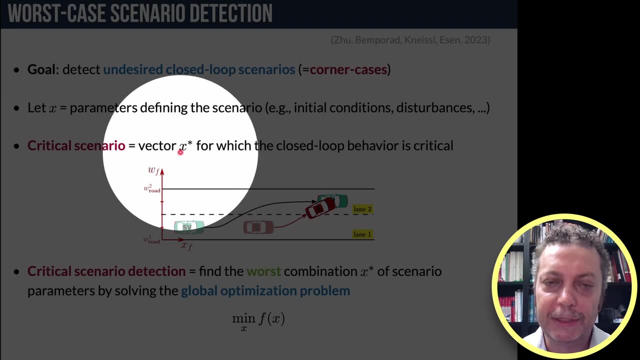 that there are no bad situations. And if there are bad situations, you may want to find those bad situations and see if they really make sense or not. So how to formulate the problem? So let's say now, x is not a vector tuning parameter. 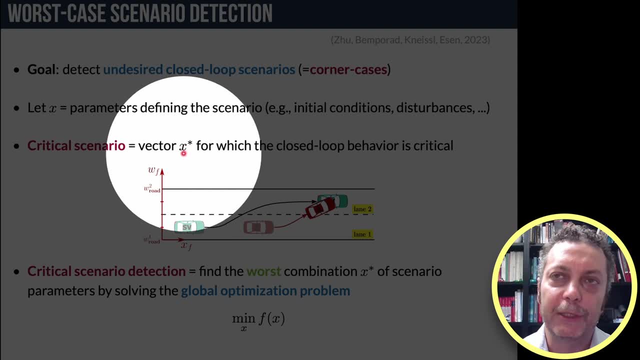 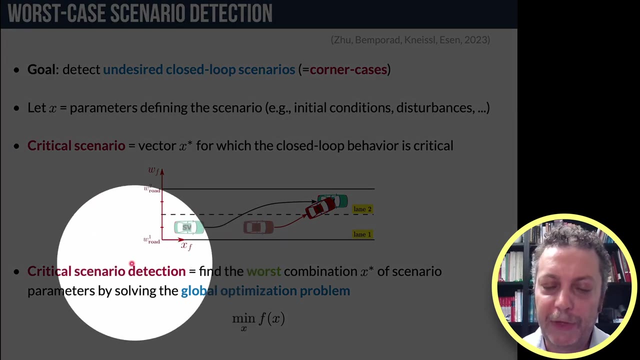 but is a vector of quantities that define a certain scenario. So, for example, it could be the initial position of the ego vehicle and the initial position and velocity of the other vehicles around you. So if you define, if you can quantify what is bad in a function f of x, 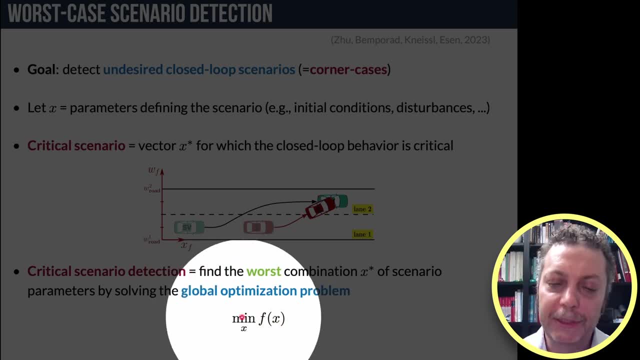 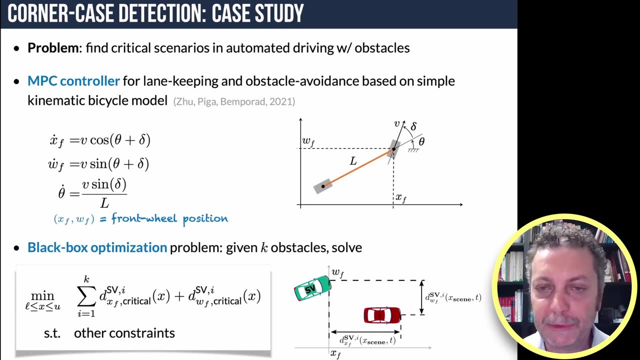 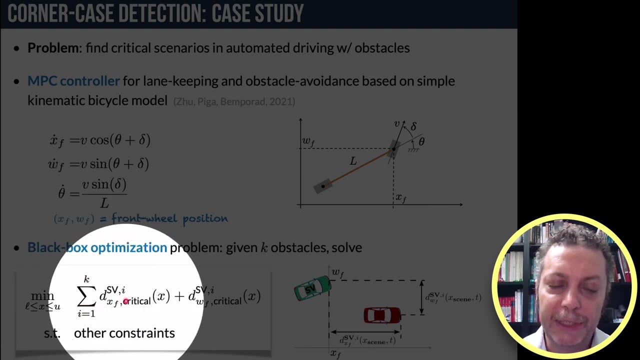 then you can minimize the function where the minimum of the function will give you the worst case you can encounter. Let me give you a concrete example. So, for the controller I was mentioning before, we define an index, which is a measure of criticality. 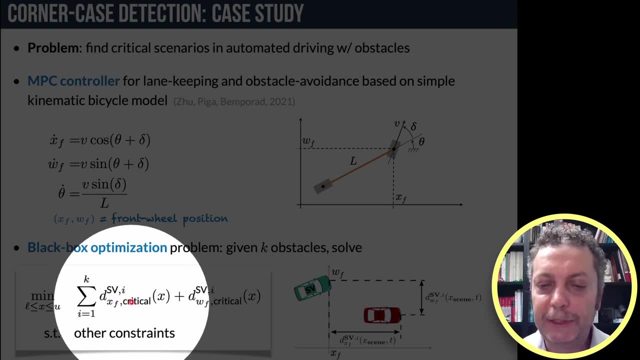 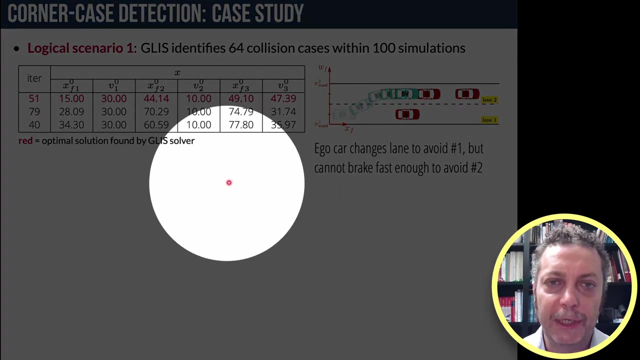 So you consider the relative longitudinal and lateral distance Between the ego vehicle and the obstacles, plus other constraints, And you optimize within certain ranges of the simulation parameters So to identify critical scenarios And in this case, for this particular setup, the software actually identifies. 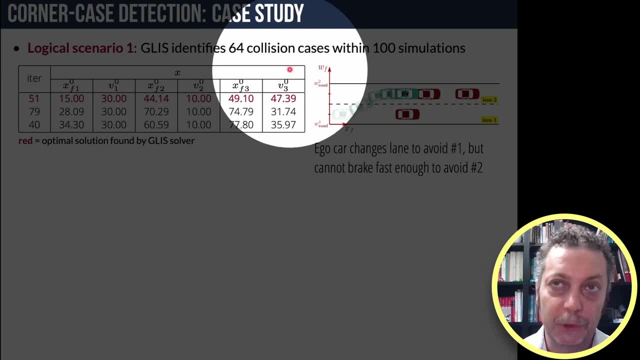 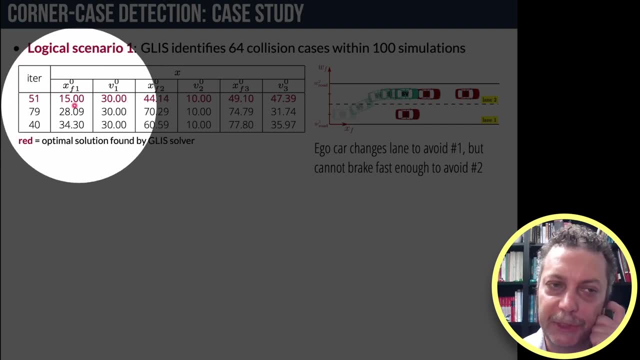 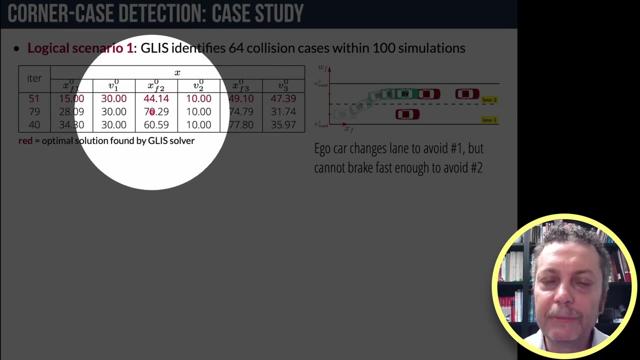 64 cases of collisions. So you will not want to want to implement that controller. Here are some results obtained, say after 51,. you get this combination of parameters determining the simulation scenario which leads to a collision, Or you can in another scenario. 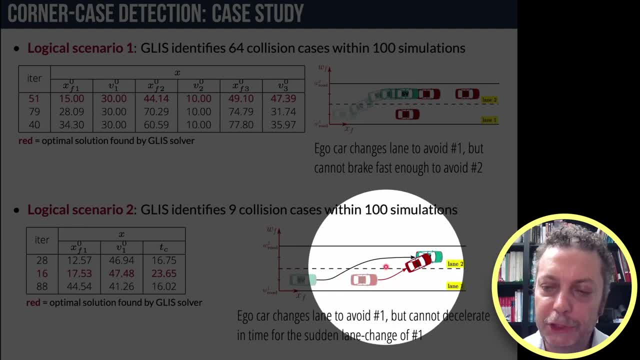 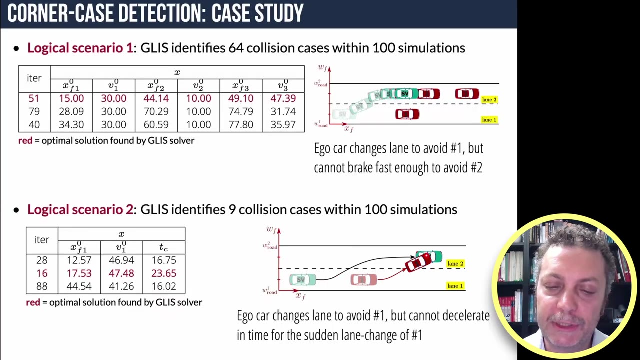 you can also allow the other vehicle to change lanes. So in this case, the software will identify a scenario where you start passing and then, meanwhile, after you start passing, the other vehicle will also change lane and you will not be able to avoid a collision.